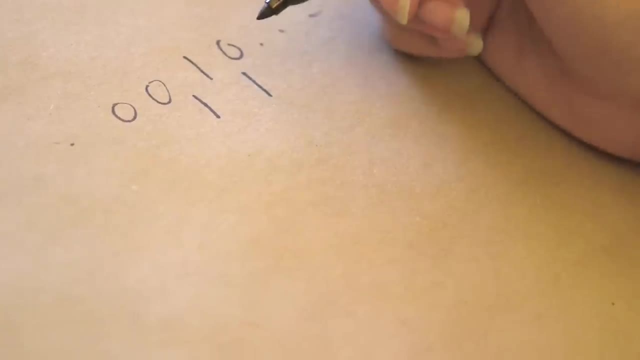 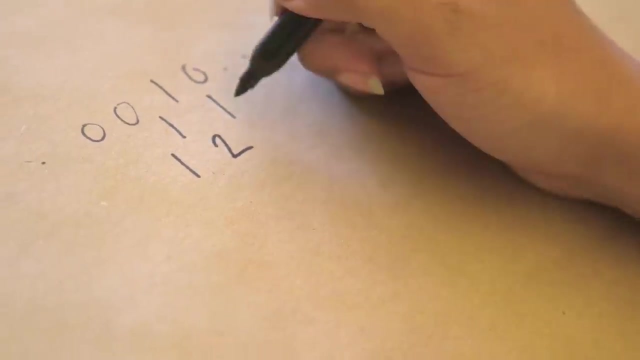 same thing on the right. All right, cool. Now I have two ones in this row and I'll do the same thing. So there's a zero we can imagine here, so we drop that down. There's one in this neighbor now, so we can have a two. And then there's one in this zero to its right, so we make another one. 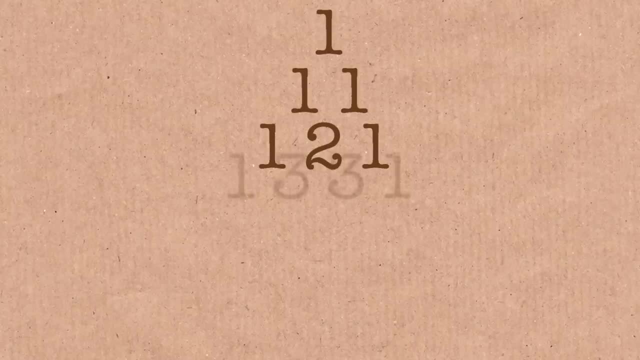 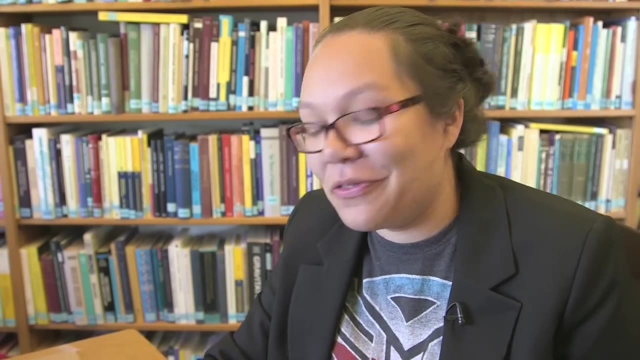 And we just keep doing this for a while And you can see that the triangle just keeps getting bigger. This isn't a thing that's going to stop. So we can just keep doing this for as long as we want. And for me, as long as I want is when the first double digit number 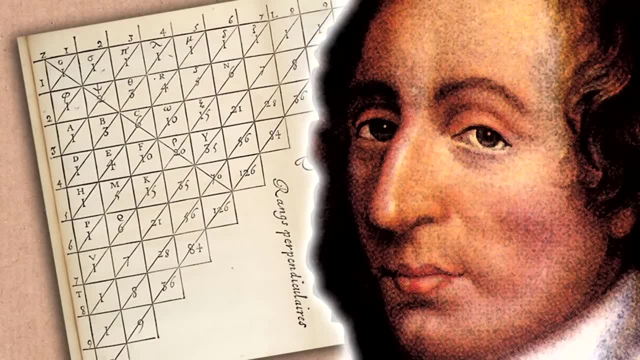 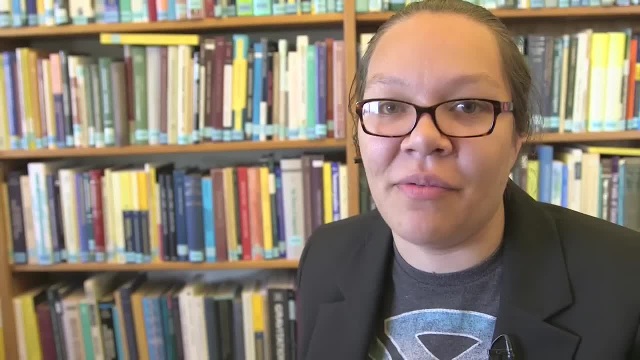 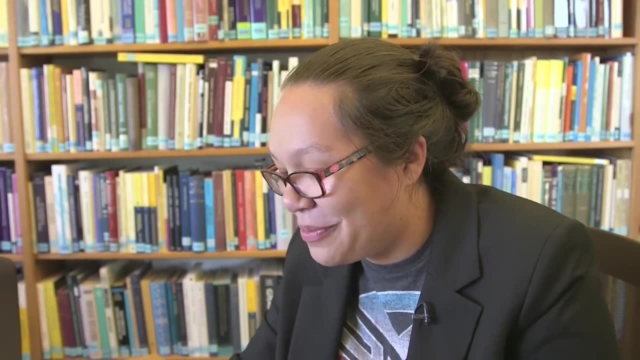 particular, Pascal was also a combinatorist. So in particular, like problems where if I have n things and I want to choose k of them, how many different ways can I do that? And it turns out that Pascal's triangle, this really like childlike adding game, as it seems to be. 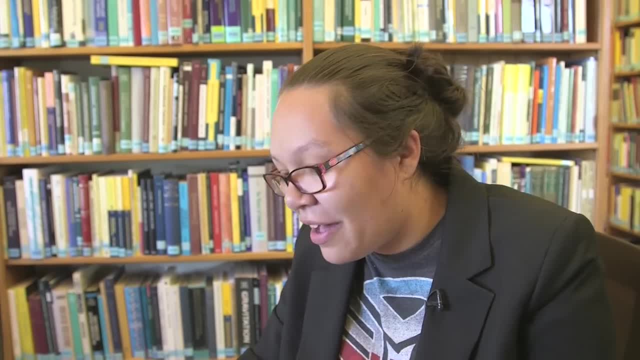 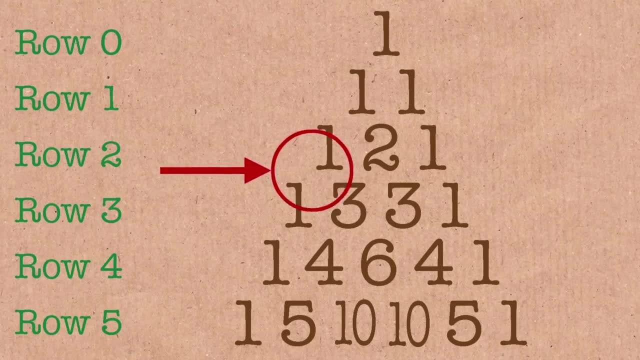 actually encodes n, choose, k. So if I have n things in particular, let's say I have four things and I want to choose, let's say one of them. then I go to the fourth row, I move over one and that's how. 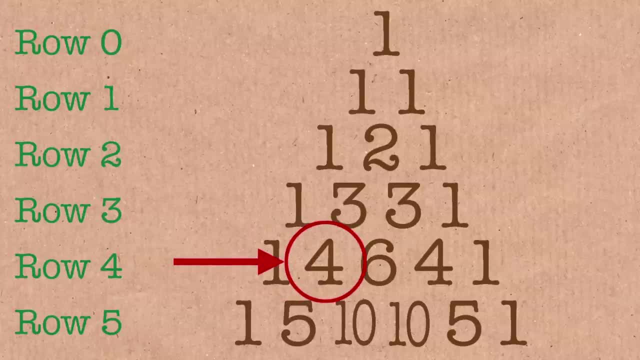 many ways I can do it, four ways. If I have four things, let's say I have like four circles and I want to only choose one of them, there are four ways I can do that. right, I can choose this one. 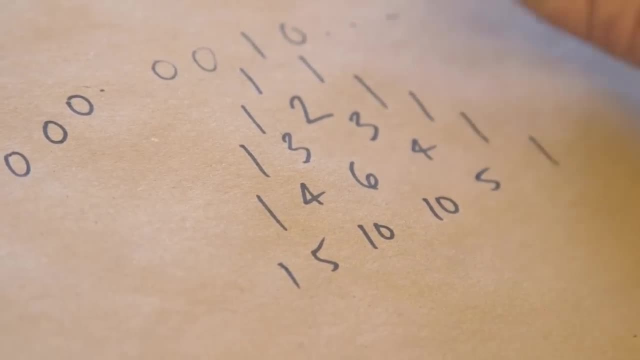 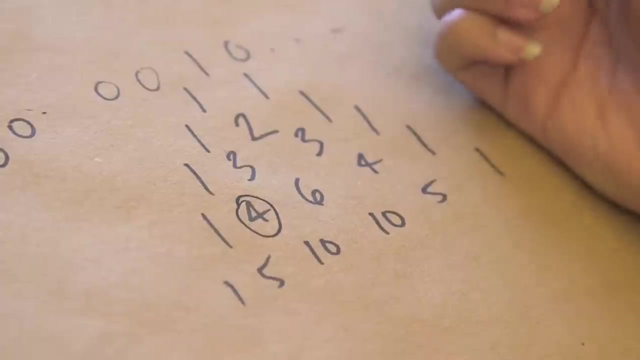 I can choose that one, I can choose that one, I can choose that one. And it turns out Pascal's triangle says: if I go down to the fourth row, where, like this is the zeroth row, and I choose one thing, so I move one over, then that's exactly how many ways I can do it. So if I told you to, 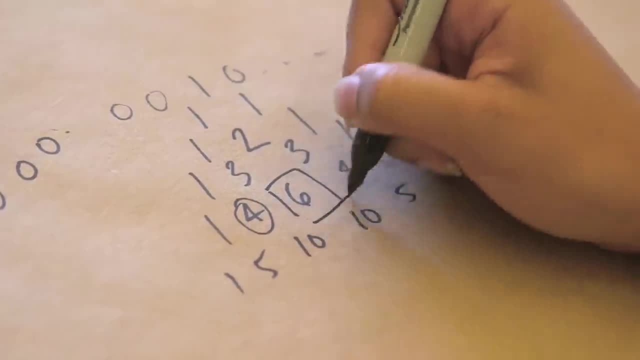 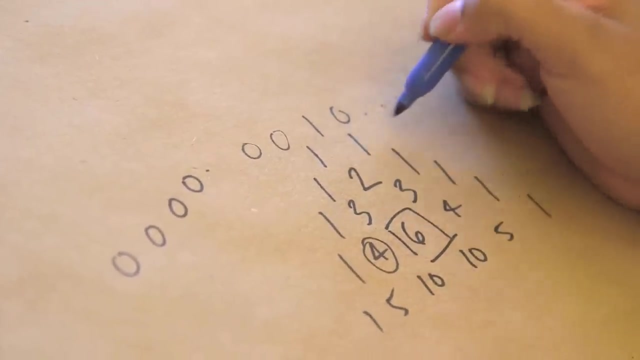 choose two circles, then there are six ways to do it. You notice that the sides are always ones like. this isn't going to change, because we just keep doing one plus zero. and then, oh look, one plus zero, one plus zero, and this is just going to keep happening. 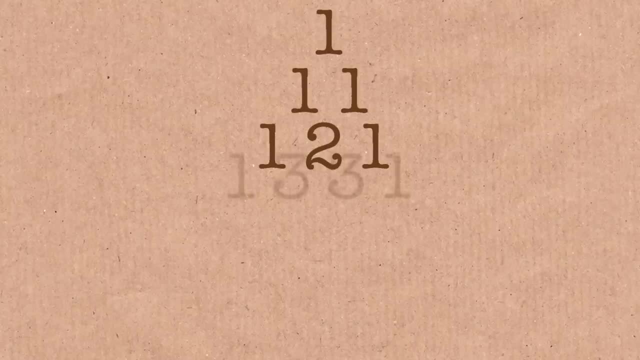 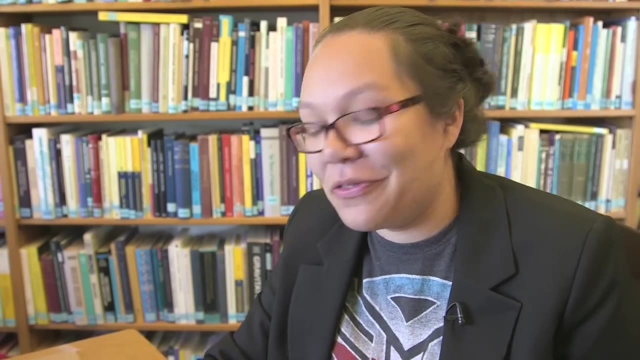 And we just keep doing this for a while And you can see that the triangle just keeps getting bigger. This isn't a thing that's going to stop. So we can just keep doing this for as long as we want. And for me, as long as I want is when the first double digit number 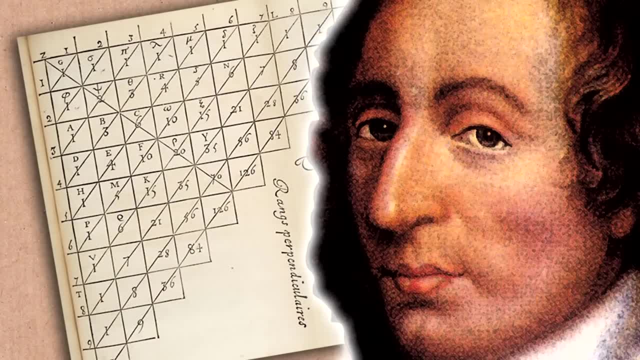 shows up because that's when adding gets hard. So Pascal was also a combinatorist. So, in particular, Pascal was a combinatorist. So, in particular, Pascal was also a combinatorist. So, in particular, like problems where if I have n things and I want to choose k of them, 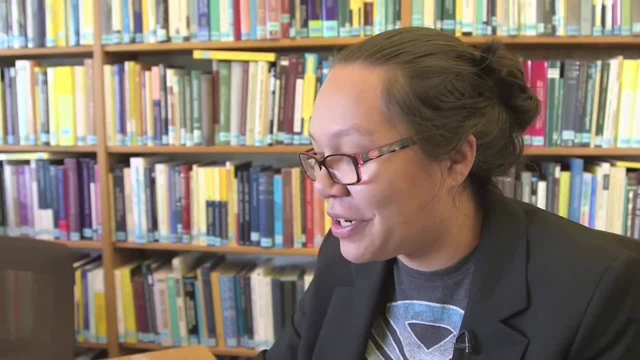 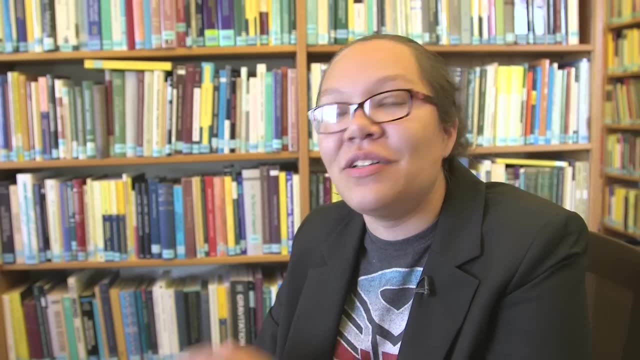 how many different ways can I do that? And it turns out that Pascal's triangle- this really like childlike adding game, as it seems to be- actually encodes n, choose k. So if I have n things in particular, let's say I have four things and I want to choose. 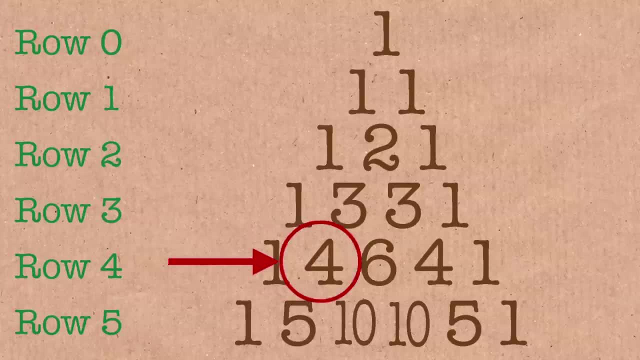 let's say one of them. then I go to the fourth row, I move over one and that's how many ways I can do it? four ways If I have four things. let's say I have like four circles and I want. 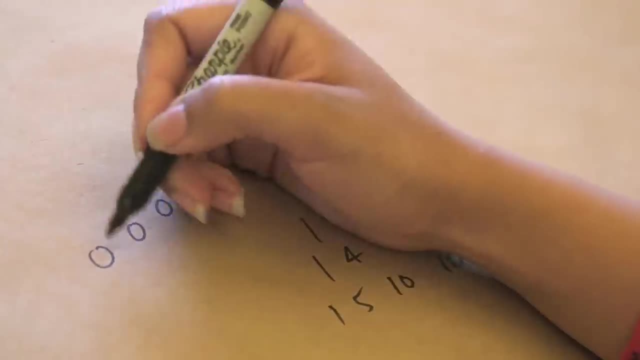 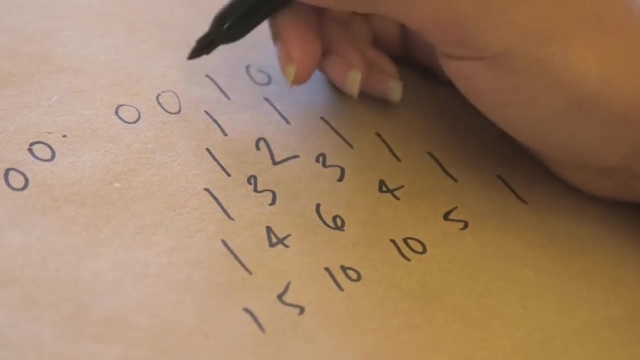 to only choose one of them. there are four ways I can do that, right. I can choose this one, I can choose that one, I can choose that one, I can choose that one. And it turns out, Pascal's triangle says: if I go down to the fourth row, where, like this, is the zeroth row and I choose, 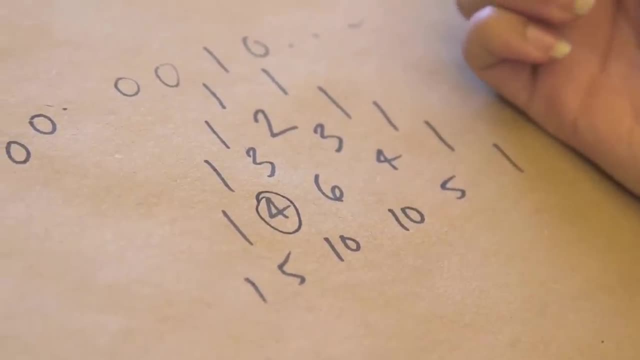 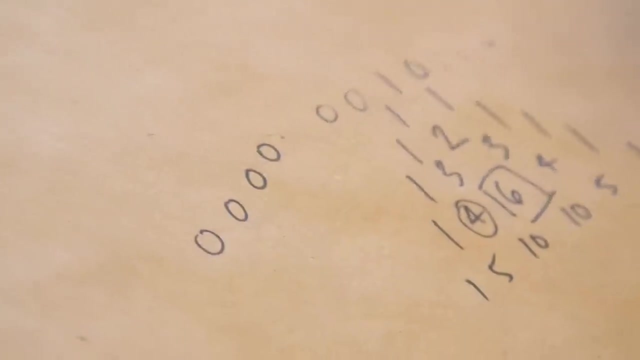 one thing, so I move one over, then that's exactly how many ways I can do it. So if I told you to choose two circles, then there are six ways to do it. You notice that the sides are always ones. Like this isn't going to change because we just keep doing one plus zero. 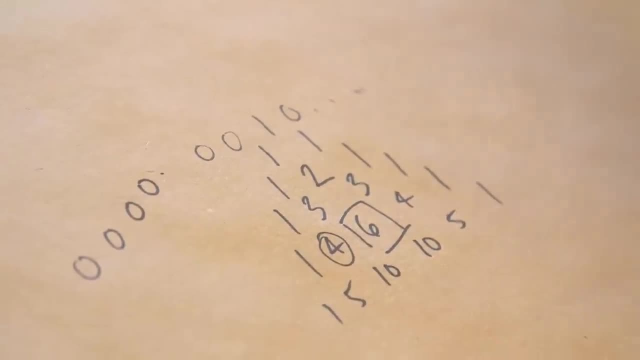 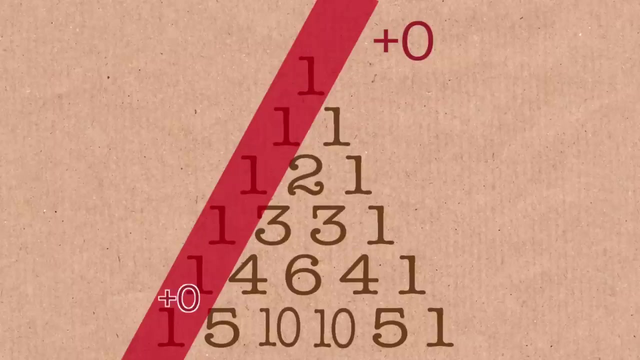 and then, oh look, one plus zero, one plus zero. And this is just going to keep happening, so we can define this entire diagonal as plus zero, because every time I go down one I'm not changing anything. But then we get to this row, right, And we have one plus one plus one. 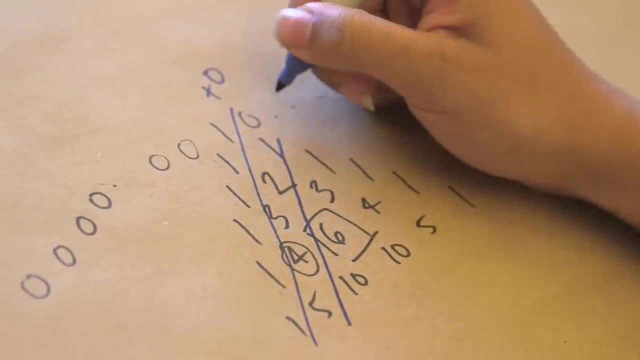 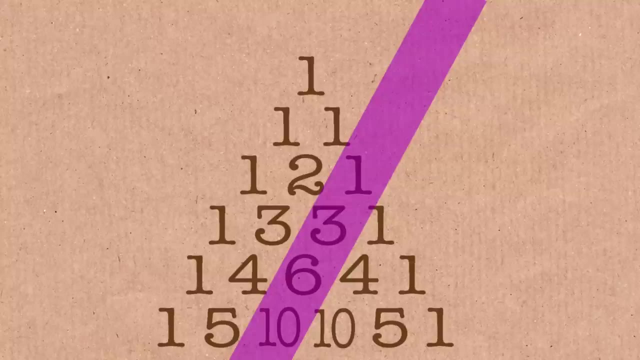 plus one, because I have zero, one, two, three, four, five, So I can define this row, if I felt like it, as plus one. Then this pattern looks less fun. right, I have one, a three, but the? 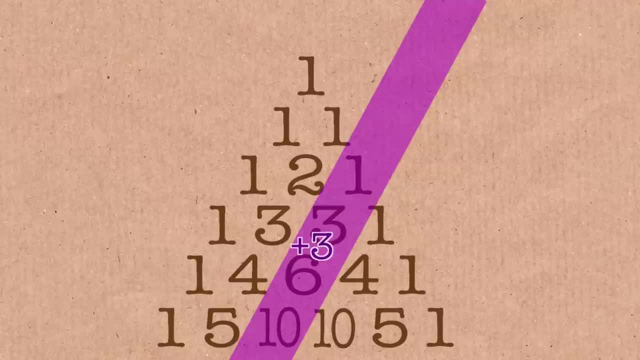 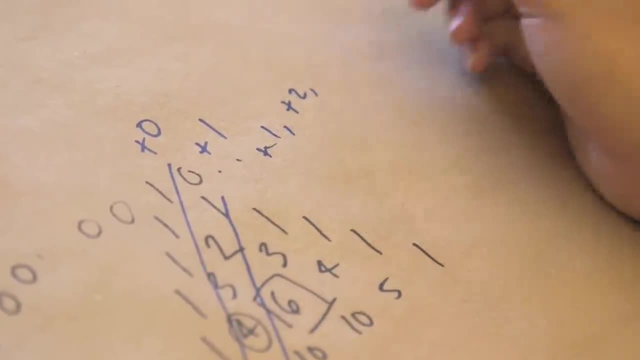 difference between three and one is two. the difference between six and three is three. the difference between ten and six is four. So it turns out this pattern is plus one, plus two, plus three. it keeps going. So around here one may be tempted to look for more patterns like: right here is like plus. 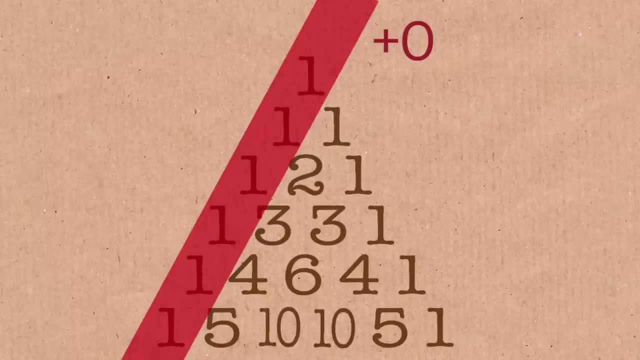 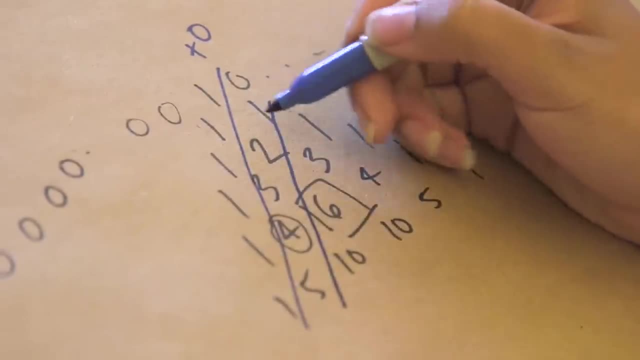 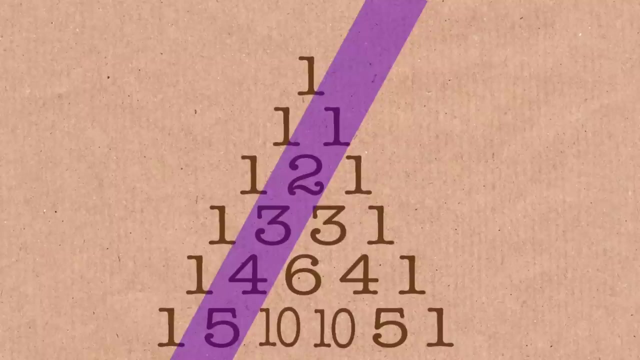 So we can define this entire diagonal as plus zero, because every time I go down one I'm not changing anything. But then we get to this row, right, And we have one plus one plus one plus one, because I have zero one, two, three, four, five. So I can define this row if I felt like it. 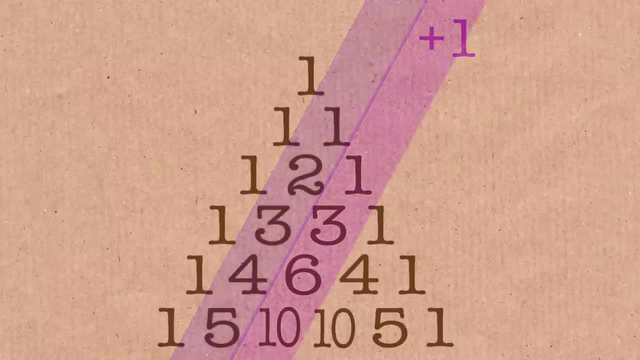 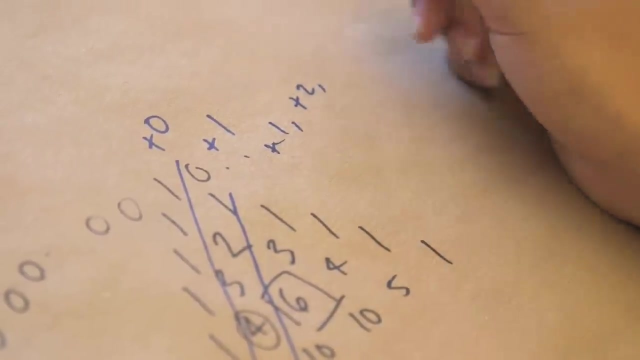 as plus one. Then this pattern looks less fun. right, I have one a three, but the difference between three and one is two. the difference between six and three is three. the difference between ten and six is four. so it turns out this pattern is plus one, plus two, plus three. 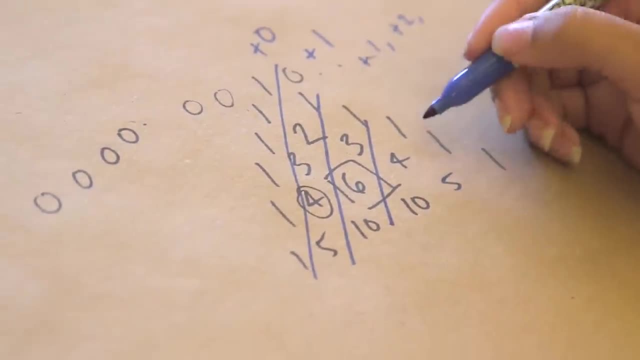 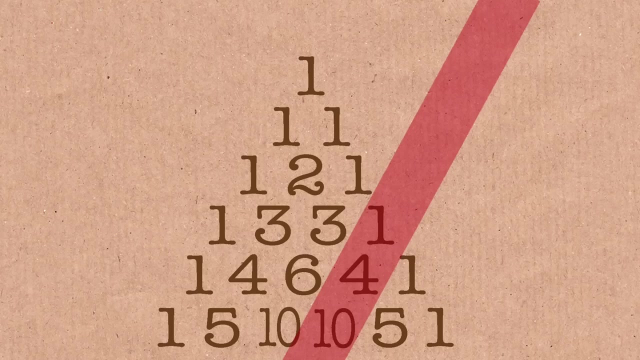 it keeps going. So around here one may be tempted to look for more patterns like right. here is like plus what? three plus six? but that's when you start to notice what we've been doing all along, which was just adding the number to the top left, like Pascal wanted us to anyway. 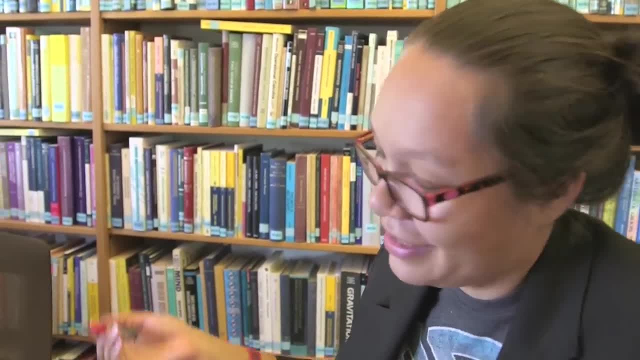 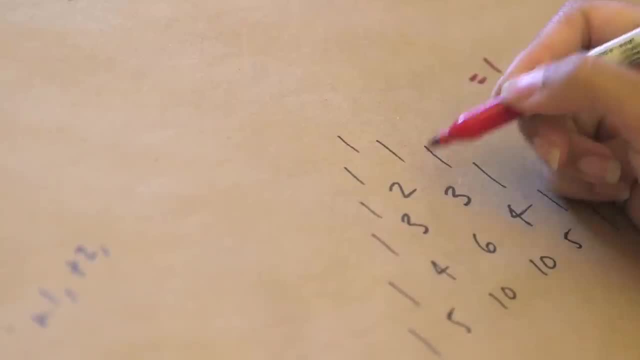 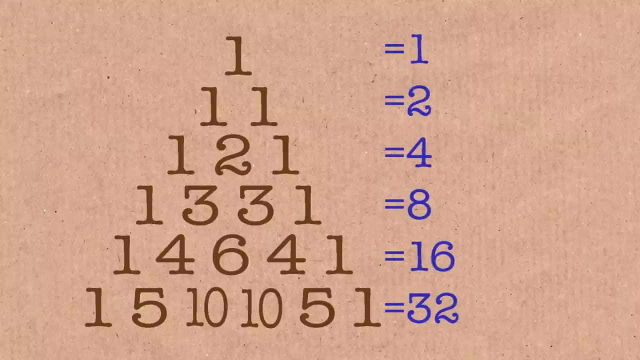 Let's just look at something else that one might be tempted to do when they see a bunch of numbers, and that's add them in a different way. So this is one. one plus one is two. one plus two plus one is four. one plus three is four plus three is seven plus one is eight. You'll notice. 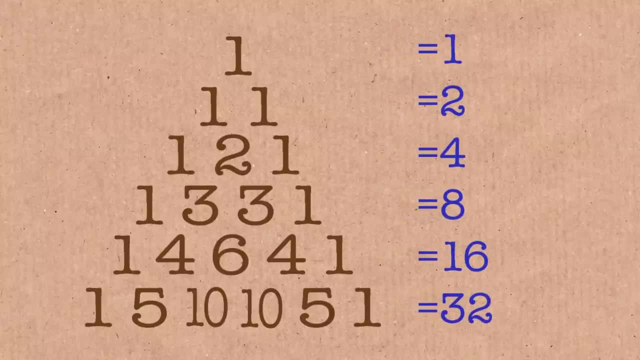 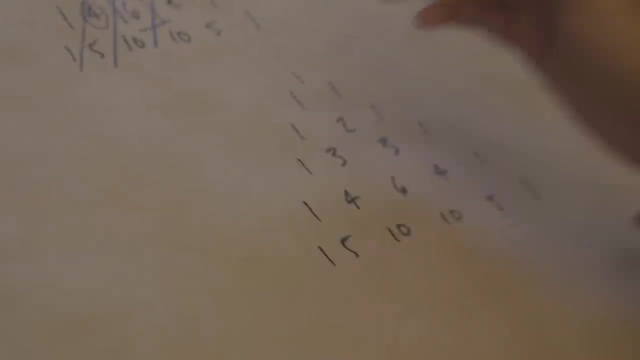 at some point. I just stopped adding because we can actually rewrite everything over here as the powers of two. So the sum of the rows of Pascal's triangle is two. like, if I'm on the nth row and I call the first one row zero, then the sum of that row is two to the n. Let's just. 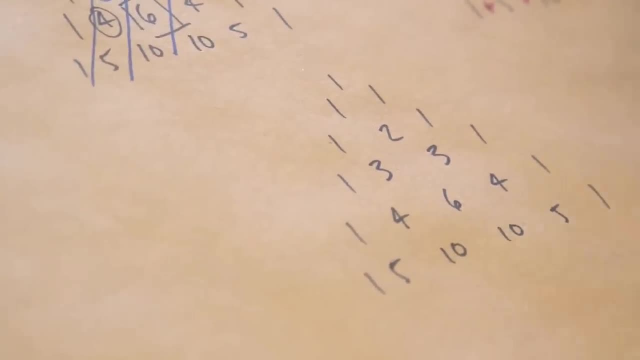 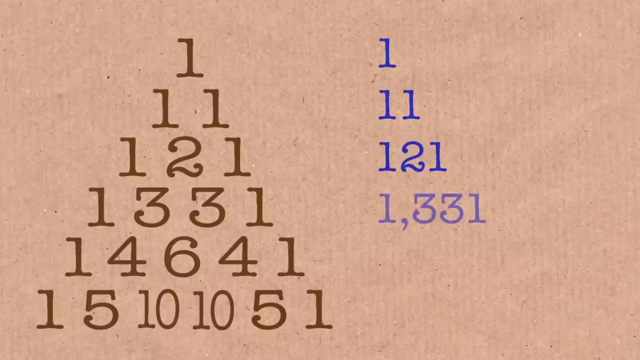 read these as numbers, let's not add them, let's not treat them as anything else. So the first row is one, the next row is eleven, the next row is a hundred and twenty-one, the next row is thirteen, thirty-one, and we get fourteen, six, four, one, and then we get to this: 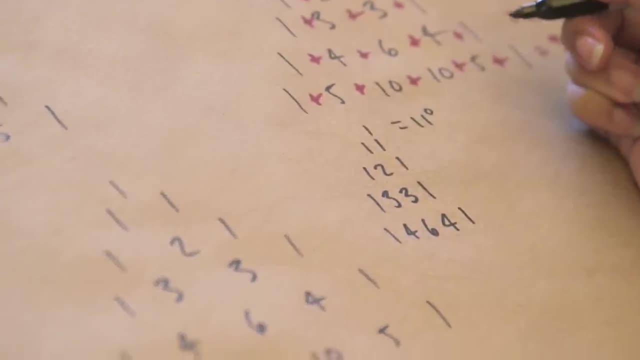 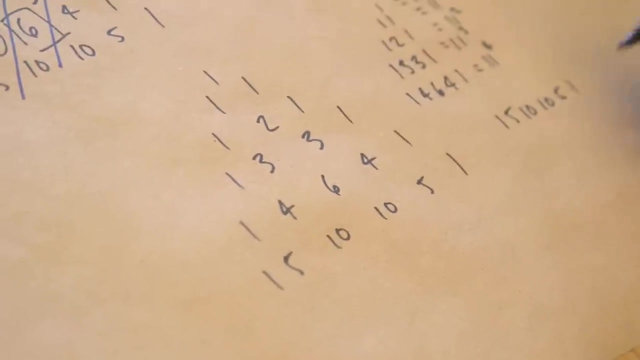 So right now these are actually the powers of eleven too. So this next row looks pretty frightening because if I wrote it out just as it is, I get a pretty big number right, Like once I put in these commas: this is around fifteen million. That's not eleven to the five, It's not 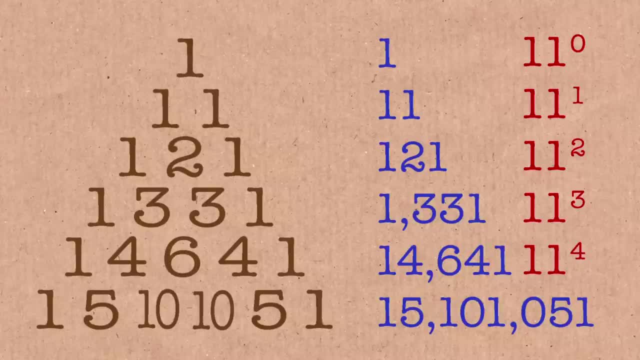 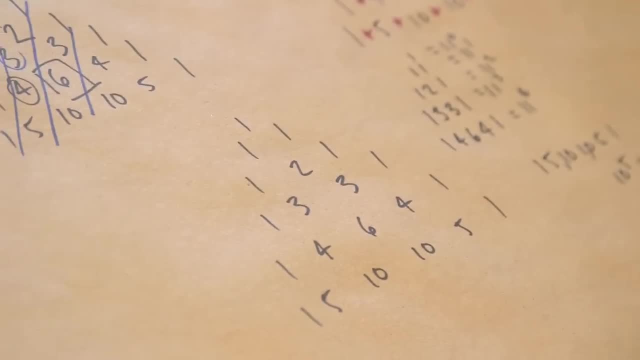 it turns out. Pascal, you know his triangle doesn't quit that early. So what's happening here is that when I was writing these as digits before, I was actually considering that place value right Like the ones place, the tenths place, the hundreds place. So I'm just going. 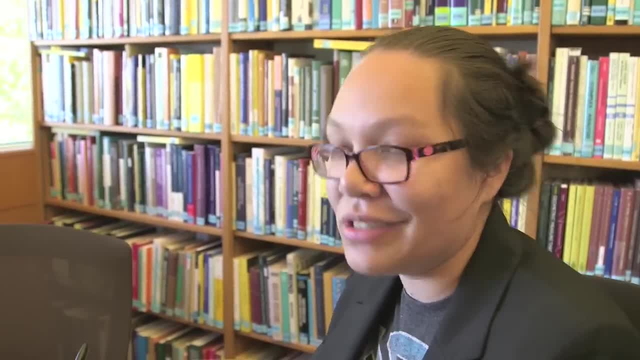 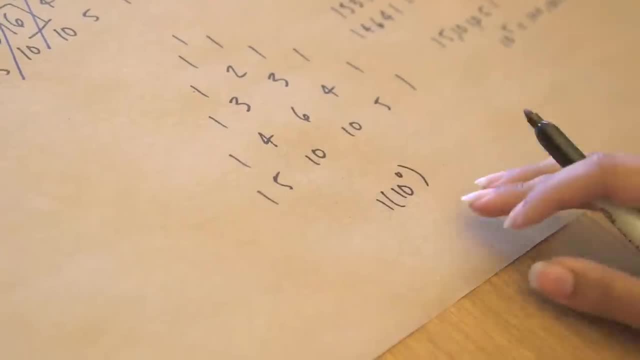 to do the same thing, where I rewrite these numbers as ones and tenths and hundreds place. So the first one will be one times ten to the zero, because this is the zeroth row. Then we have one times ten to the one plus one times ten to the zero. 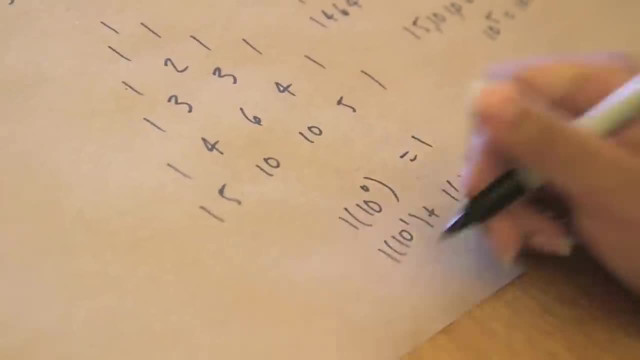 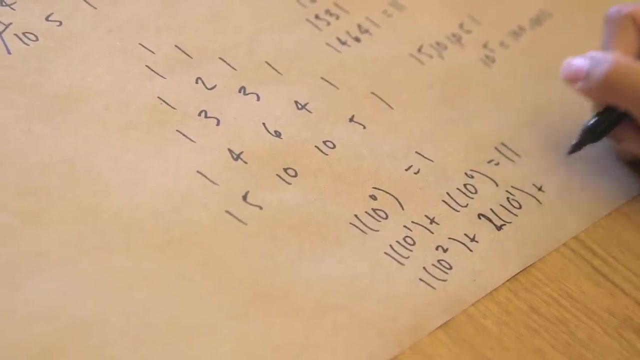 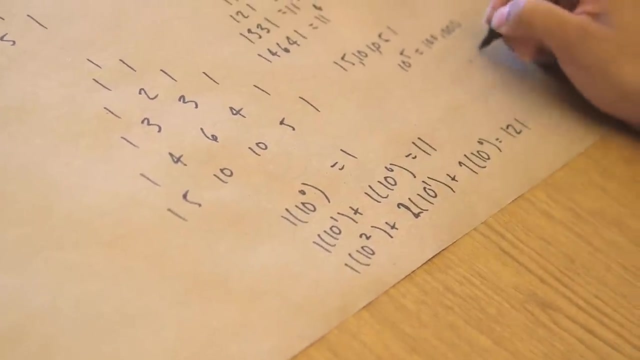 So this one's one, this one's eleven. Let's do one times ten squared plus one times ten, two times ten to the one- my bad- plus one times ten to the zero, That's a hundred and twenty-one. So let's skip on down to our friend. here We do one times ten to the five plus. 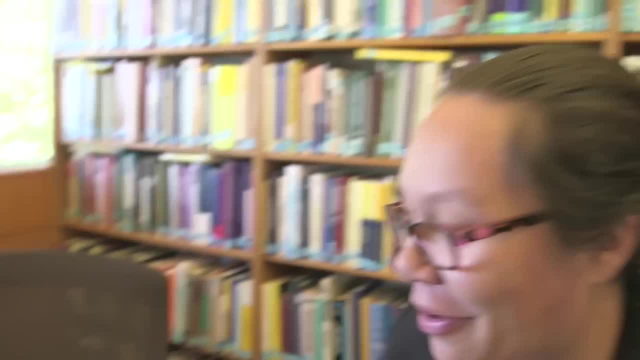 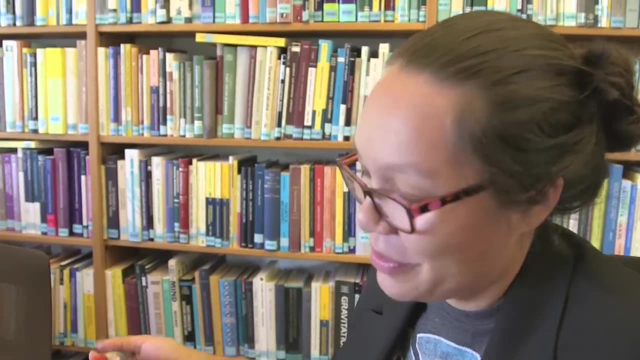 what three plus six. But that's when you start to notice what we've been doing all along, which was just adding the number to the top left, like Pascal wanted us to. anyway, Let's just look at something else that one might be tempted to do when they see a bunch of numbers. 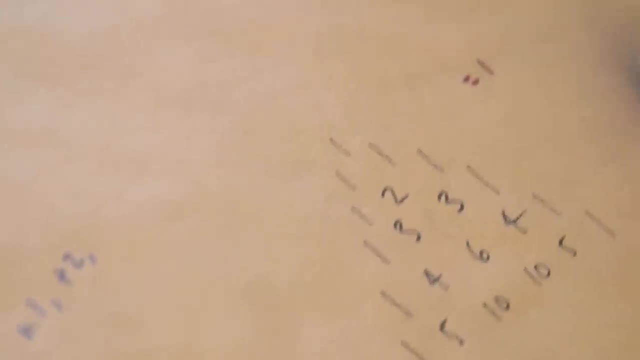 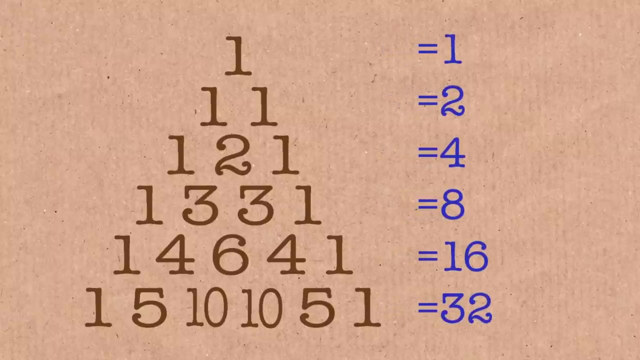 and that's add them in a different way. So this is one. one plus one is two. one plus two plus one is four. one plus three is four plus three is seven plus one is eight. You'll notice, at some point I just stopped adding because we can actually rewrite everything over. 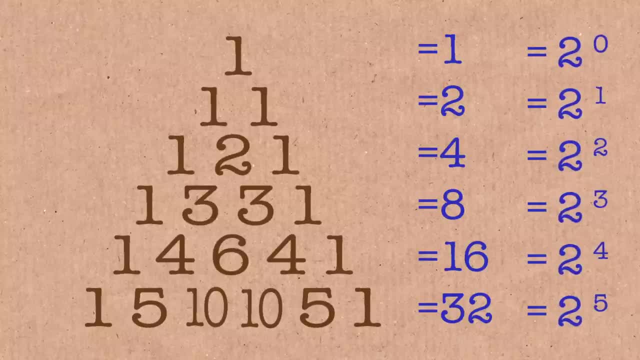 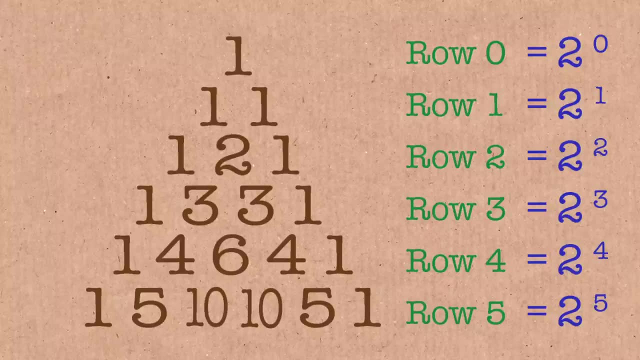 here as the powers of two. So the sum of the rows of Pascal's triangle is two. like, if I'm on the nth row and I call the first one row zero, then the sum of that row is two to the n. Let's just 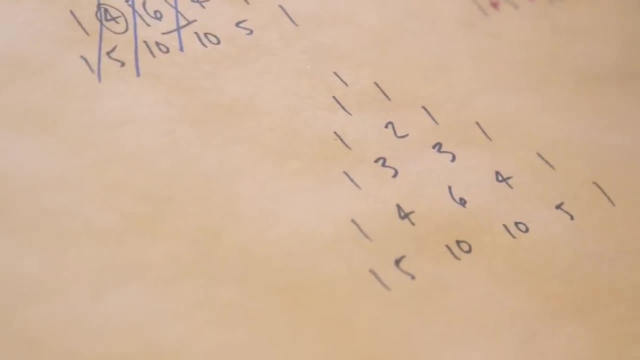 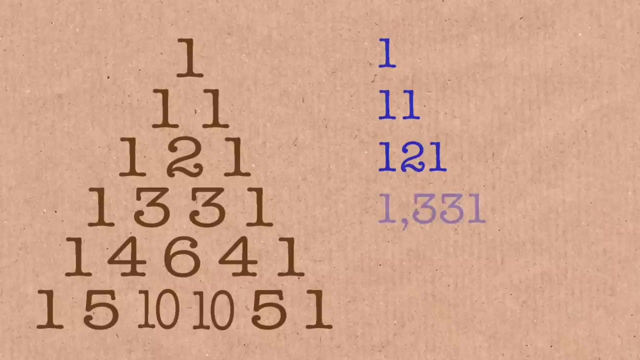 read these as numbers, let's not add them, let's not treat them as anything else. So the first row is 11,, the next row is 121,, the next row is 1331, and we get 14641,, and then we get to this: 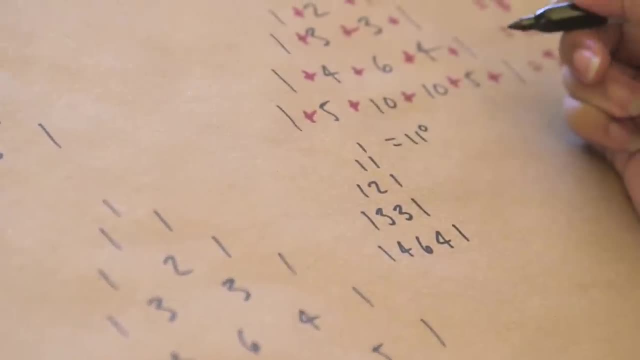 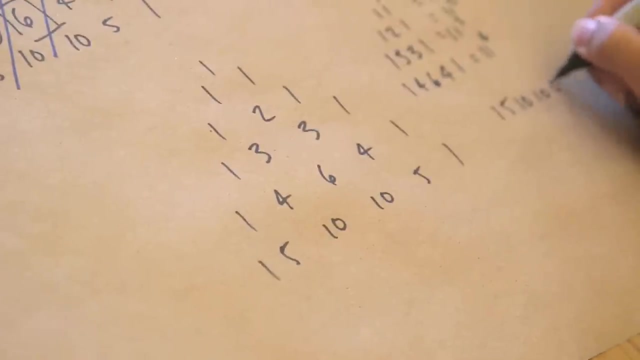 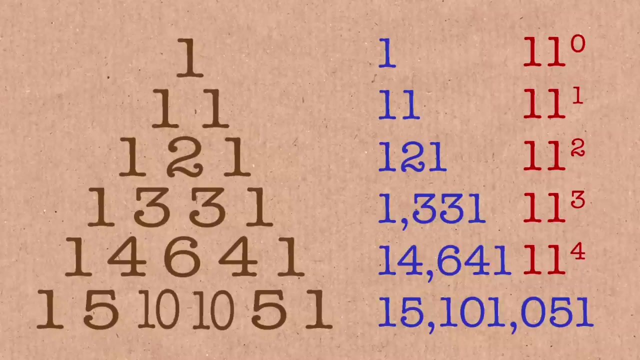 So right now, these are actually the powers of 11 too. So this next row looks pretty frightening because if I wrote it out just as it is, I get a pretty big number right. Like once I put in these commas: this is around 15 million. That's not 11 to the 5. It's not, But it turns out, Pascal, you know. 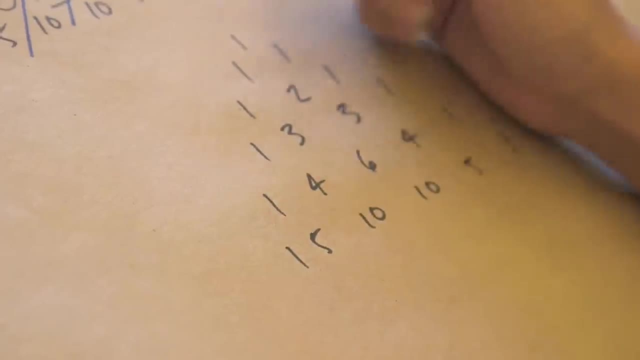 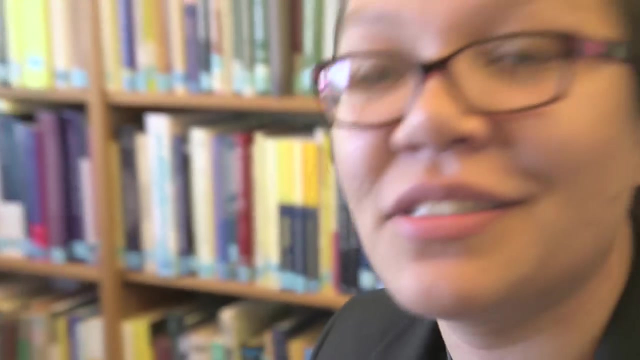 his triangle doesn't quit that early. So what's happening here is that when I was writing these as digits before, I was actually considering that place value right, Like the ones place, the tenths place, the hundredths place. So I'm just going to do the same thing where I rewrite: 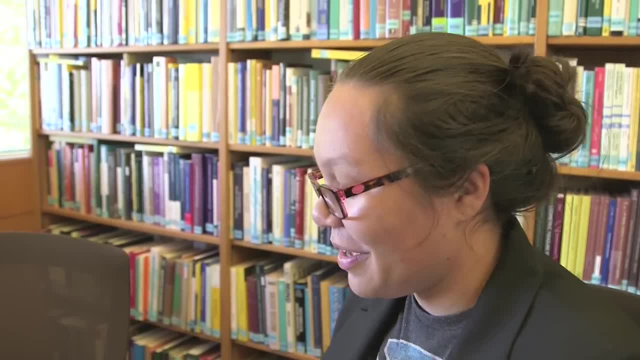 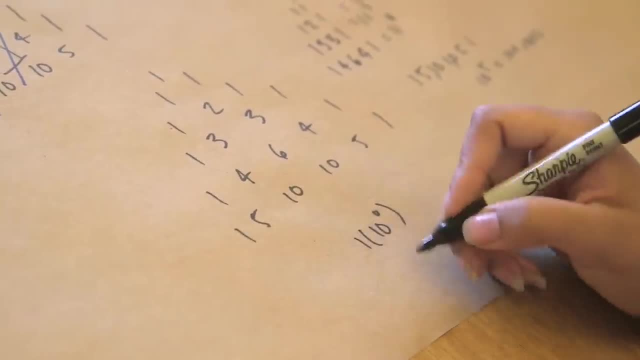 these numbers as ones and tenths and hundredths place. So the first one will be 1 times 10 to the zero, because this is the zeroth row. Then we have 1 times 10 to the 1, plus 1 times 10 to the zero. 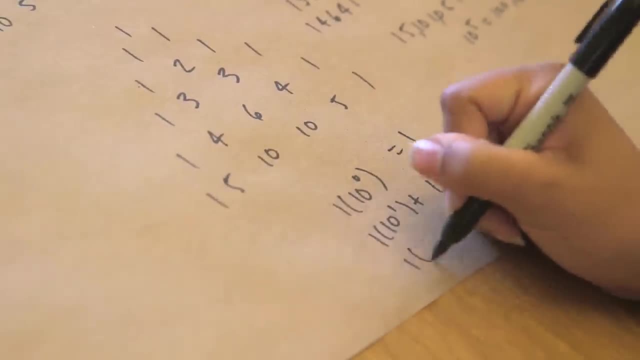 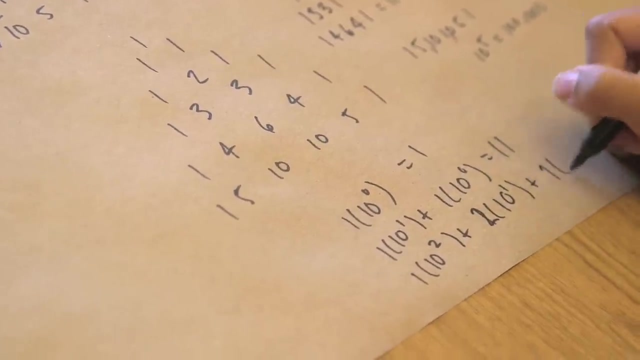 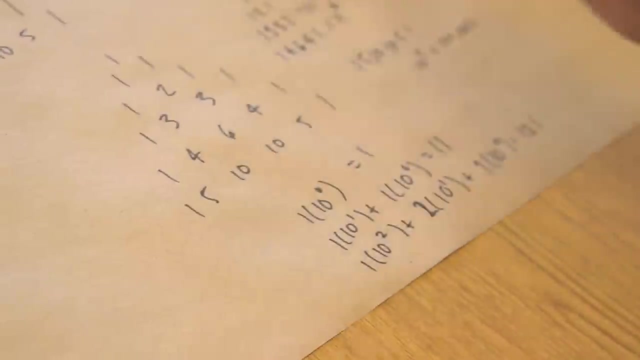 This one's 11.. Let's do 1 times 10 squared plus 1 times 10, oh, 2 times 10 to the 1, my bad. plus 1 times 10 to the zero, That's 121.. So let's skip on down to our friend here. 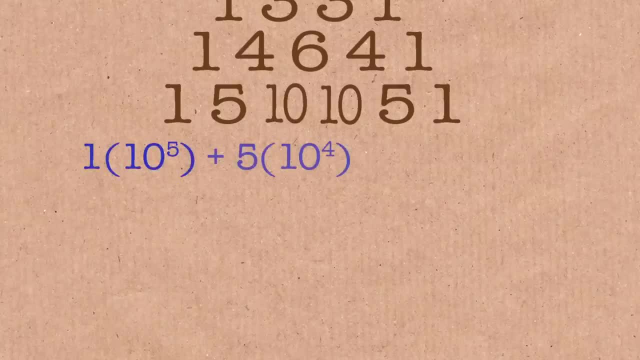 We do 1 times 10 to the 5 plus 5, 10 to the 4 plus 10 to the 3 plus 10. squared, Yeah, 5 to the 10 to the 1 and 1 times 10 to the zero, And this is 11 to the 5.. 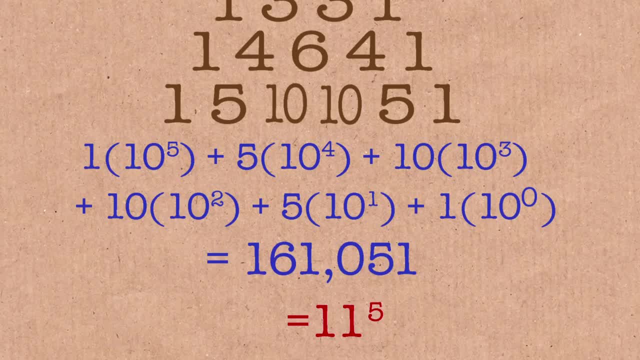 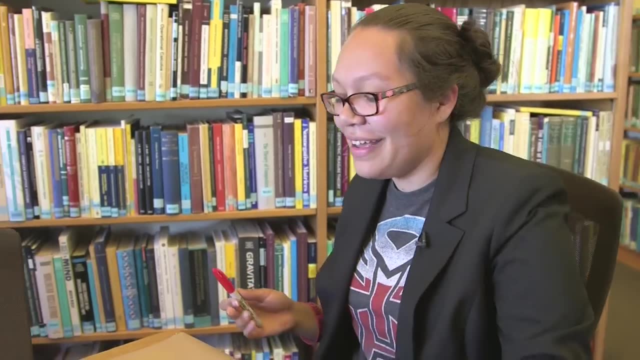 So it is 11 to the 5.. It is 11 to the 5.. It's just hiding. So now I have this really cool thing that I found extremely recently called the hockey sticks method- I think some people call it. It's just a really cool trick. 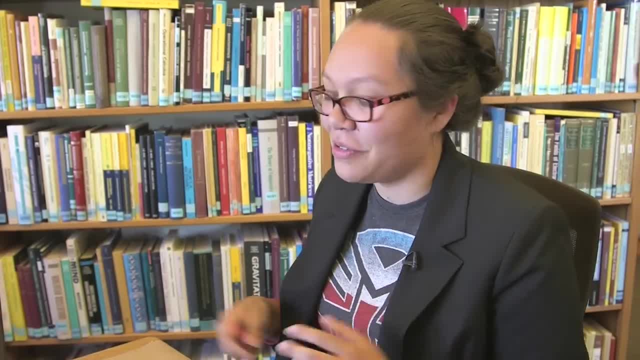 that you can do on Pascal's triangle- Another result of the fact that it's the coefficients of like a binomial expansion. So it's just a really cool trick that you can do on Pascal's triangle- Another result of the fact that it's the coefficients of like a binomial expansion. 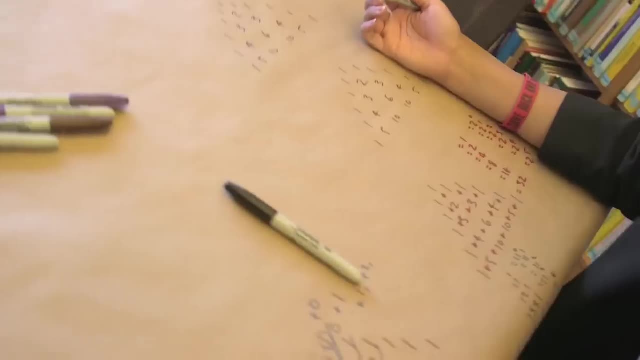 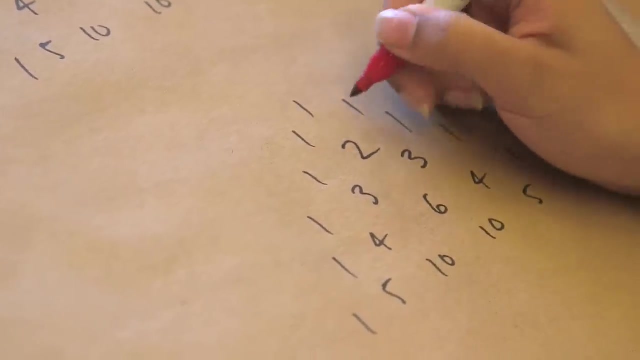 Which is all a. it will make more sense once I draw a hockey stick. What you do is you pick a 1 somewhere on the edge and you just go down diagonally. So I'm going to pick this 1 and then I'm going to go down diagonally, and then I'm just going to keep going and then at. 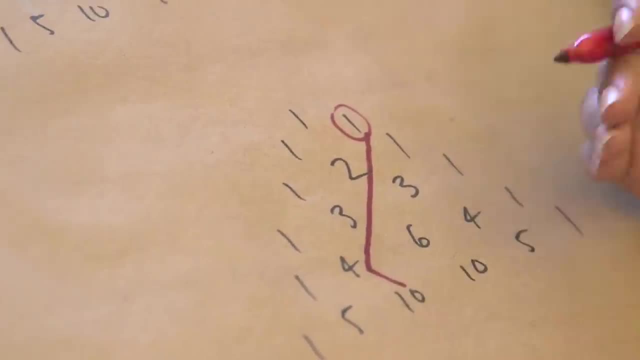 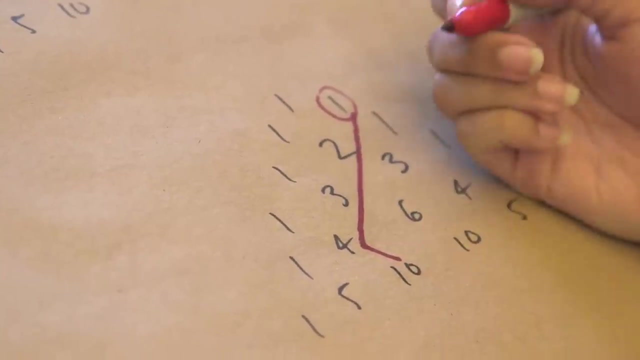 some point. I'm just going to veer off. In this case I have to veer off because I didn't draw any more rows, So the number that I veer off to is the sum of all the numbers I trace down. 1 plus 2 plus 3 plus 4 equals 10.. So this row 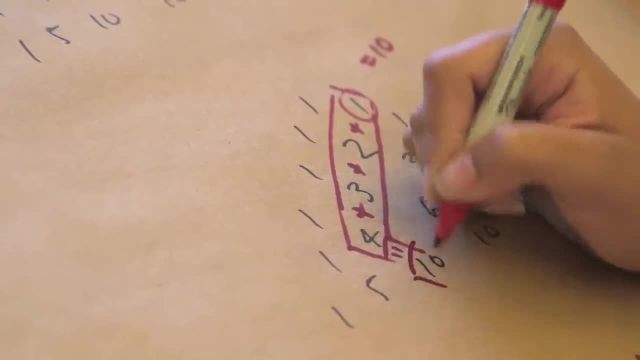 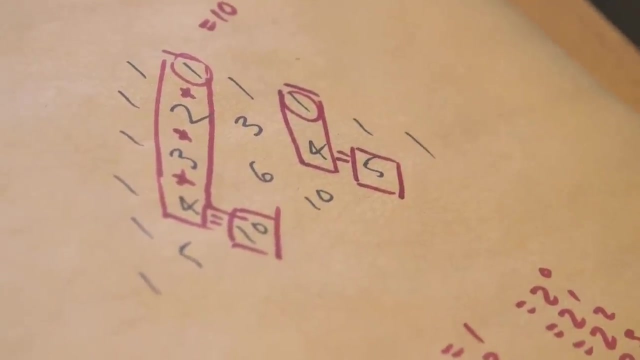 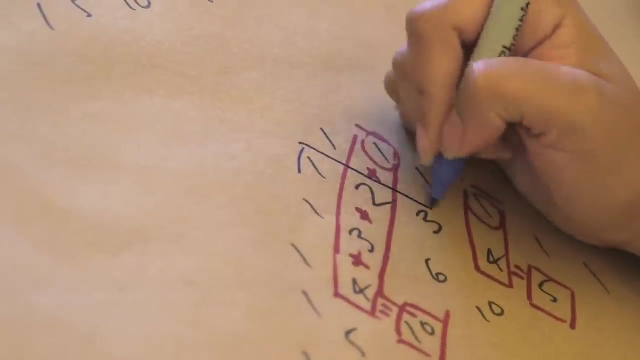 or this diagonal rather equals 10.. So I'm going to start with this one and I'm just going to veer off real quickly. actually I'm just going to all right. So it works on small ones. Let's use this one because- why not? We can do the other direction right. 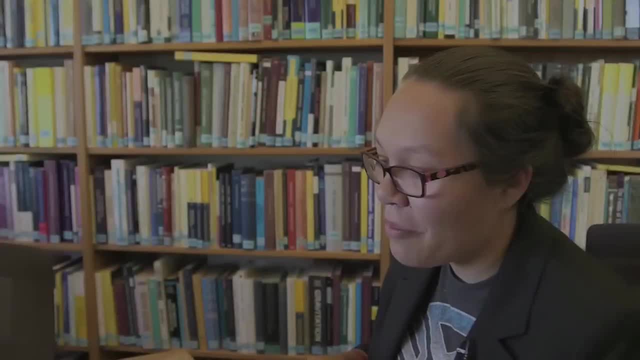 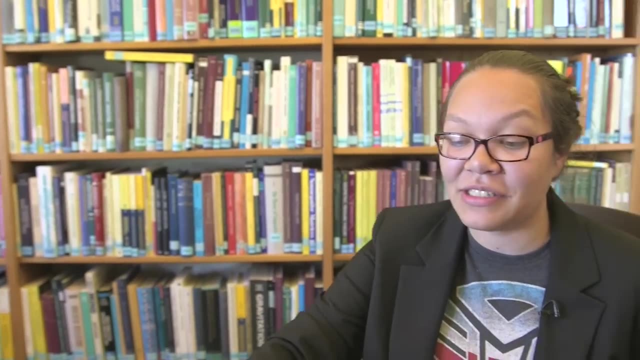 and we get 1 plus 2 plus 3 equals 6.. I'm going to do Pascal's triangle, mod 2.. So, brief aside, mod 2 in this case is just going to mean that every time a number is odd, I write it as a 1. 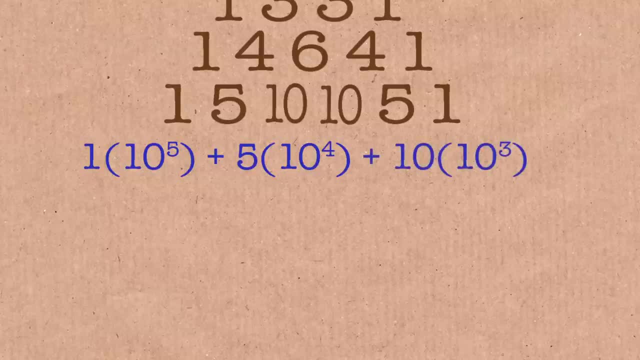 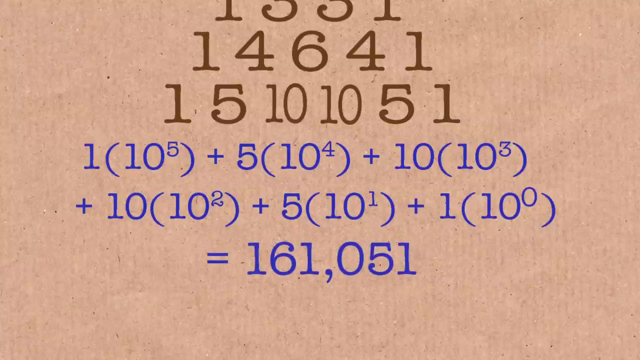 five, ten to the four plus ten to the three plus ten. ten squared, yeah, five to the ten to the one and one times ten to the zero, And this is eleven to the five. So it is eleven to the five. 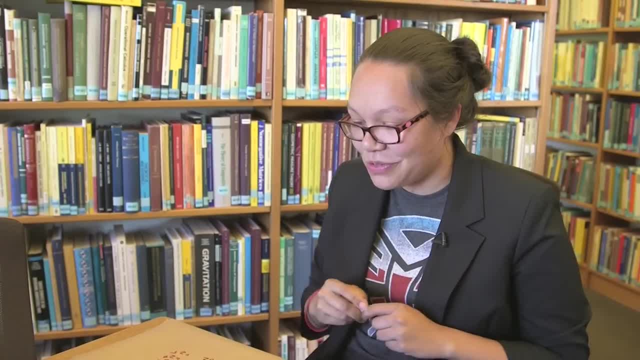 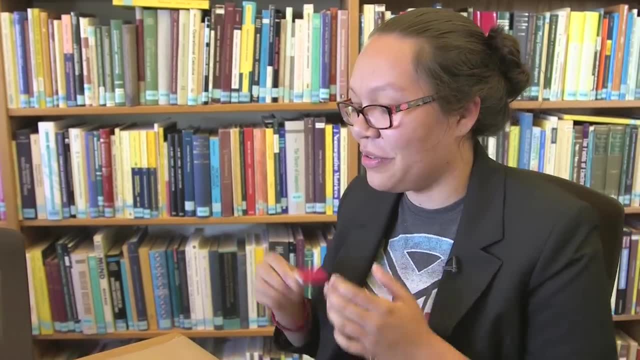 It is eleven to the five. it's just hiding. So now I have this really cool thing that I found extremely recently called the hockey sticks method, I think some people call it. It's just a really cool trick that you can do on Pascal's triangle, another result of the fact that 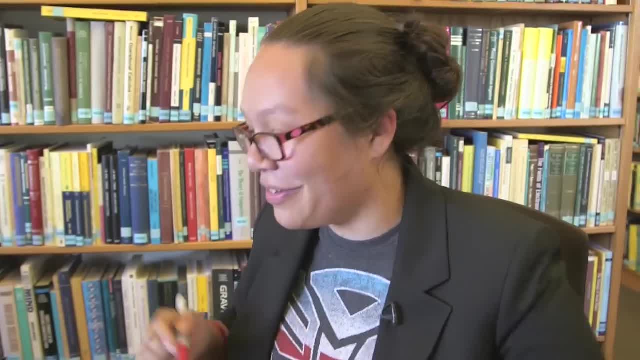 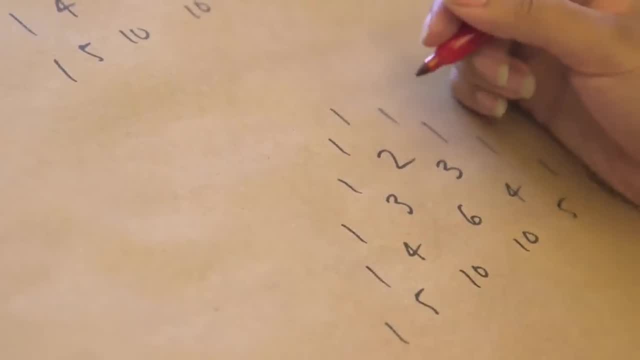 it's the coefficients of a binomial expansion, which is all a. It will make more sense once I draw a hockey stick. What you do is you pick a one somewhere on the edge and you just go down diagonally. So I'm going to pick this one and then I'm going to go down diagonally. 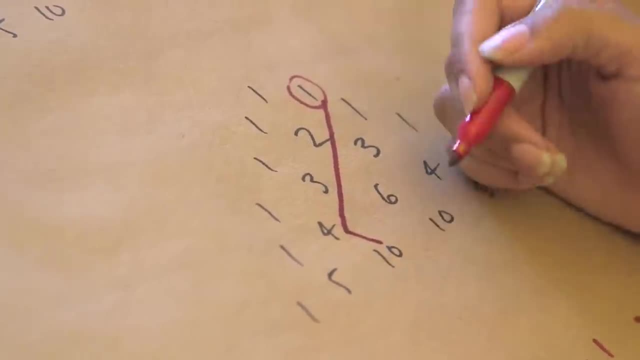 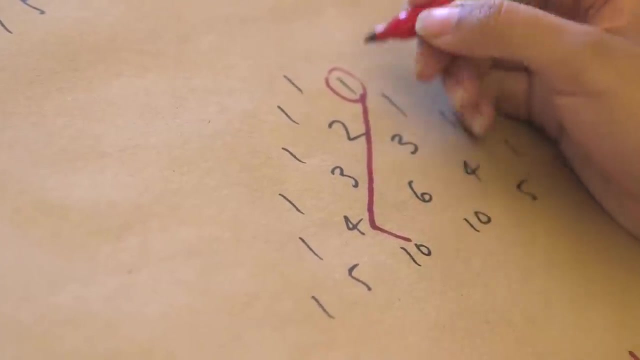 and then I'm just going to keep going and then at some point I'm just going to veer off. In this case I have to veer off because I didn't draw any more rows, So the number that I veer off to is the sum of all the numbers I traced down: One plus two plus three. 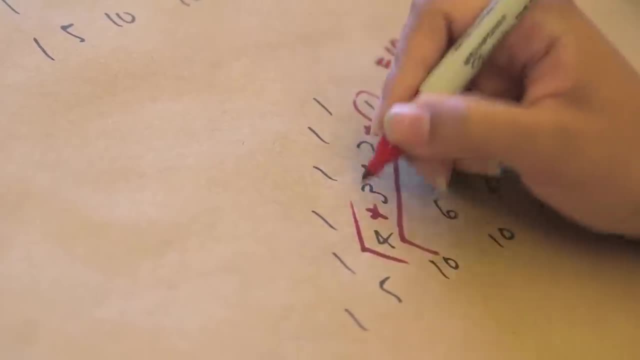 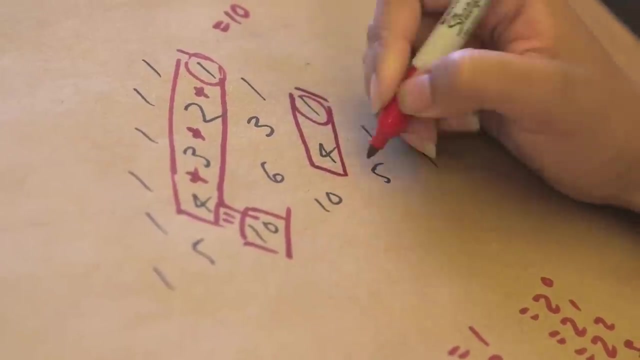 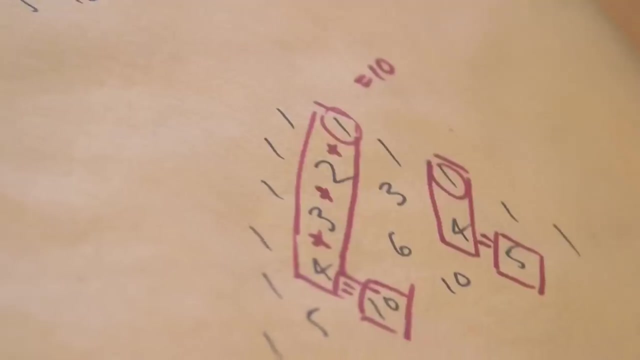 equals ten. So this row or this diagonal, rather equals ten. So I'm going to start with this one and I'm just going to veer off real quickly. actually I'm just going to. Alright, So it works on small ones. Let's use this one because- Why not? We can do. 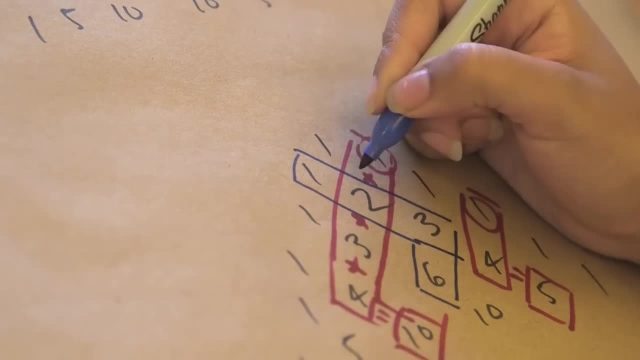 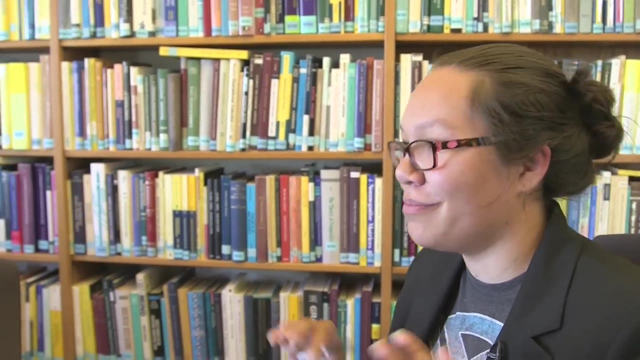 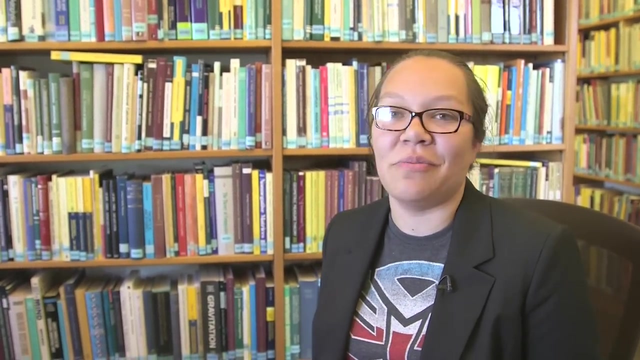 the other direction right, And we get one plus two plus three equals six. I'm going to do Pascal's triangle, mod two. So, brief aside, mod two, in this case, is just going to mean that every time a number is odd, I write it as a one, and every time a number is even, I write it as a zero. 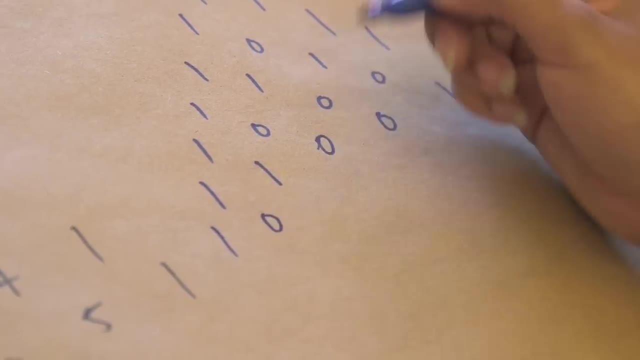 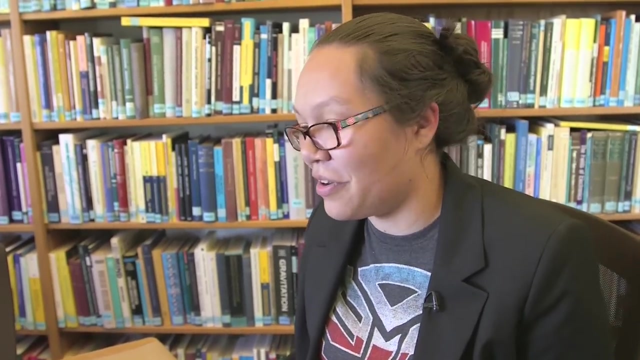 Cool, Cool right, That's still a Pascal triangle, is it? Yeah, just mod two. It doesn't like preserve the actual value of the numbers as much, but it totally tells you whether or not something's even or odd, and that's all we care about right now. So then I'm going to outline all of the 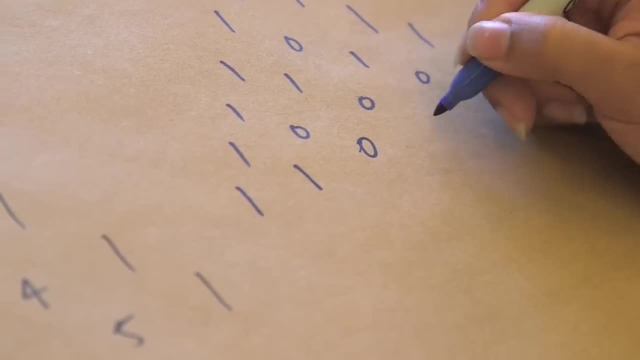 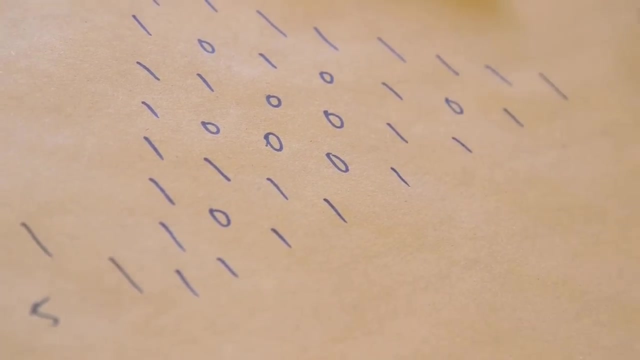 and every time a number is even, I write it as a 0.. Cool right, That's still a Pascal triangle, is it? Yeah, just mod 2.. It doesn't like preserve the actual value of the numbers as much, but it totally tells you whether or not something's even or odd, and that's all we care about right now. So then, 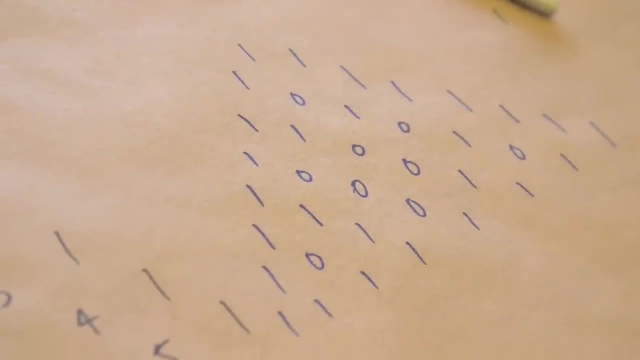 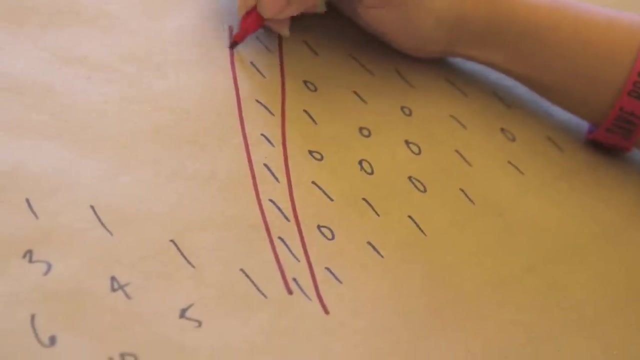 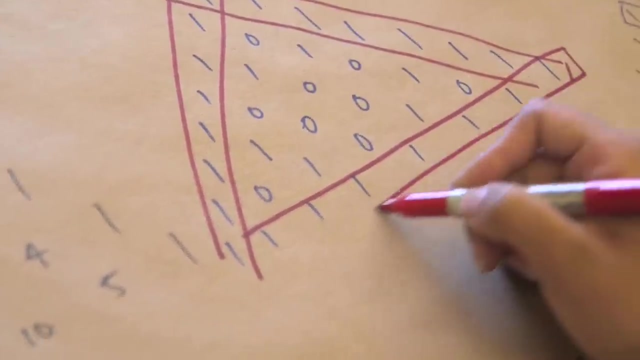 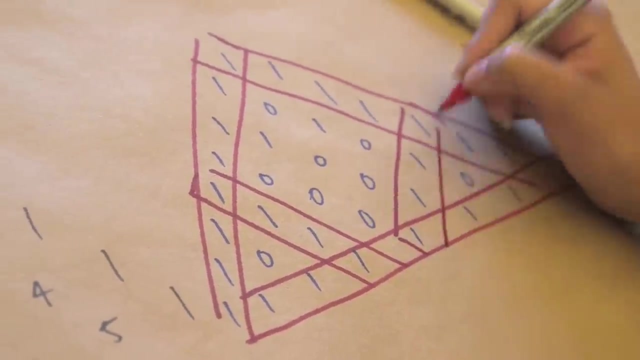 I'm going to outline all of the diagonals- that are all ones- and all the rows- that are all ones. So I'm gonna do this, Which isn't the world's prettiest thing, but it's pretty nice, And this shape should maybe start to look a little familiar if you've played. 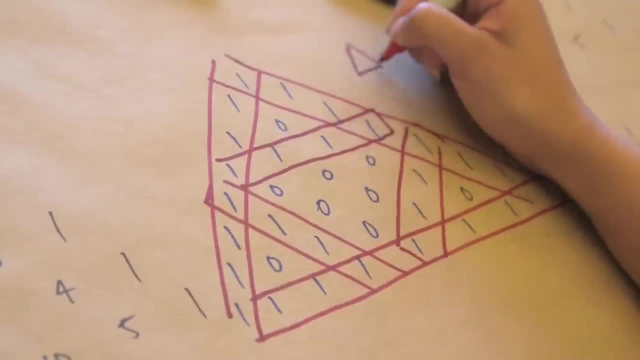 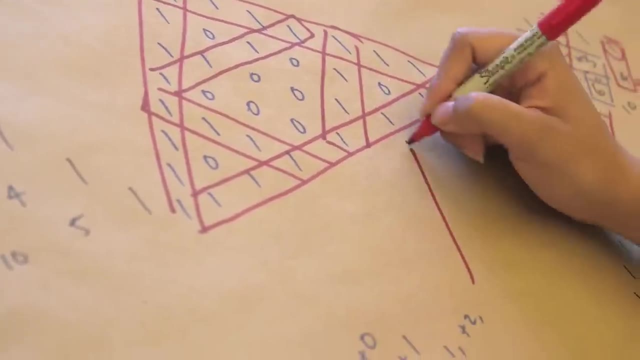 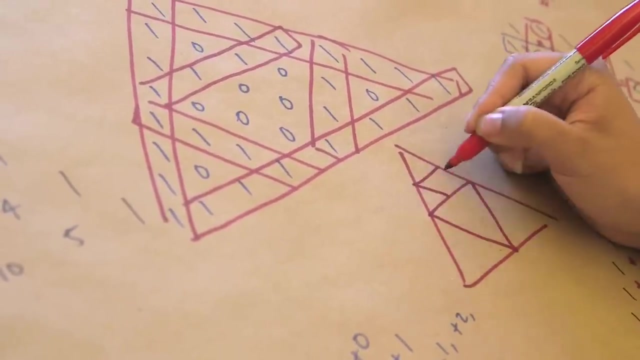 Legend of Zelda. before It's also the Triforce, but more importantly, it's Sierpinski's triangle. So for those who don't recognize Sierpinski's triangle, I start with an equilateral triangle, I inscribe another one upside down, and then I can just keep doing this on all of the 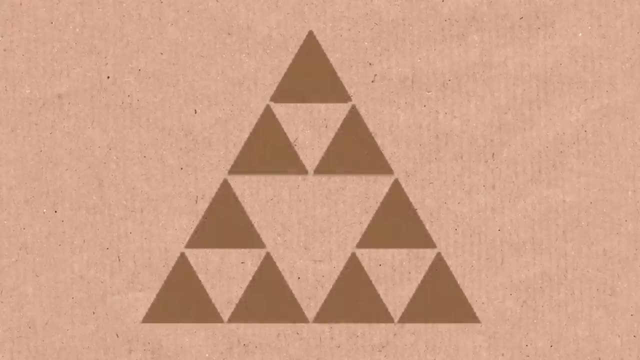 upward, facing triangles as many times as I want. So yeah, this can just go on for a long time. Cool, And it turns out that the way that the evens and odds show up in Pascal's triangle when I convert them to mod 2, I can make Pascal's triangle as big as I want, and I'm just going. 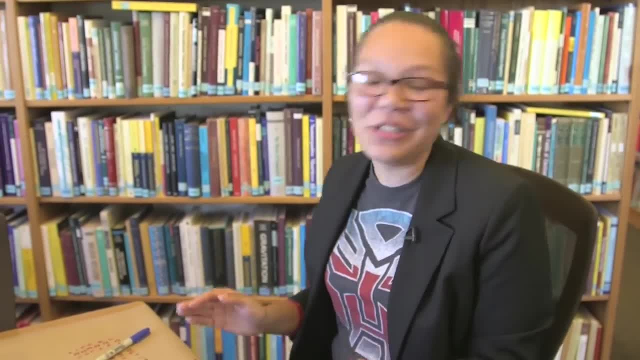 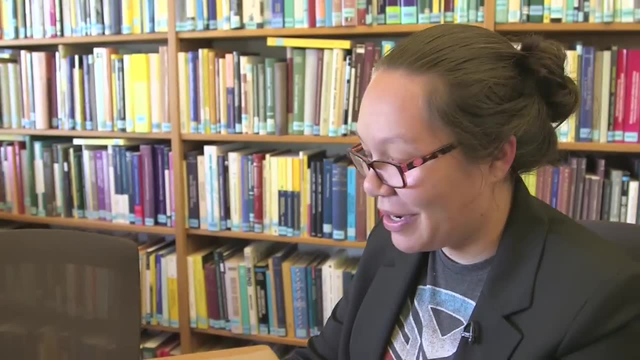 to keep getting iterations of Sierpinski's triangle. So that's really cool, That's awesome. It's really cool by itself, but it's also a good rule to follow. But it gets cooler using the mod2 construction. There's something else we can do in mod2, though. 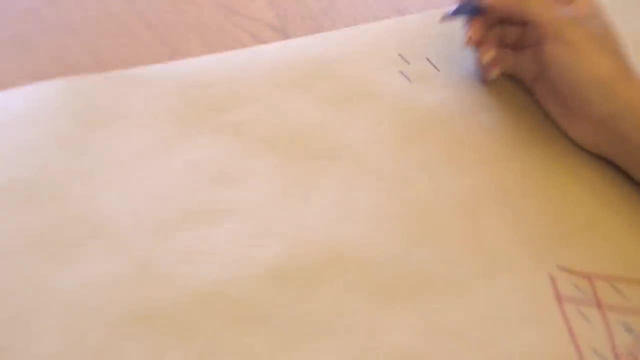 In particular, we can write down the same things, but let's write them now, as We've got 1s and 0s right And for most people, 1s and 0s kind of remind them of binary. 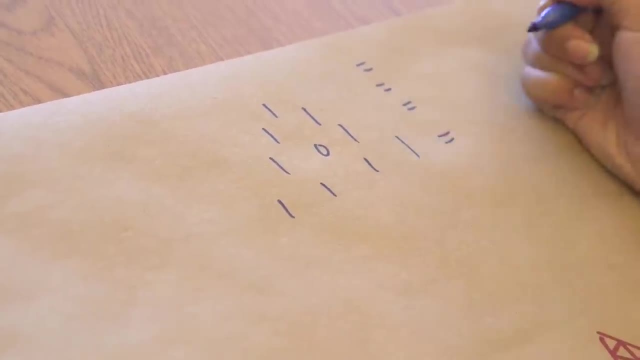 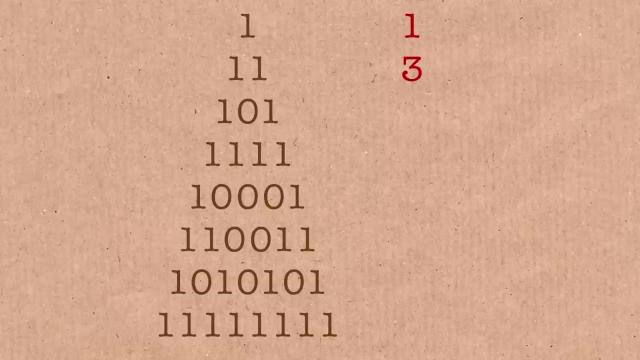 So let's just see what happens when we transcribe these from binary. You know, 1 in binary 1. And then 1, 1 in binary is 3.. 1,, 0, 1 is 5.. 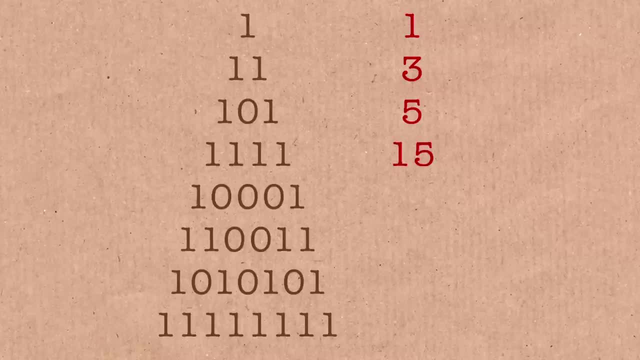 1, 1, 1 is 15.. And then the next one: 1, 0, 0, 0, 1 is 17.. Now, these may not immediately appear pretty cool, But if I kept going, the next one is 51,, the next one is 85,, after that is 255. 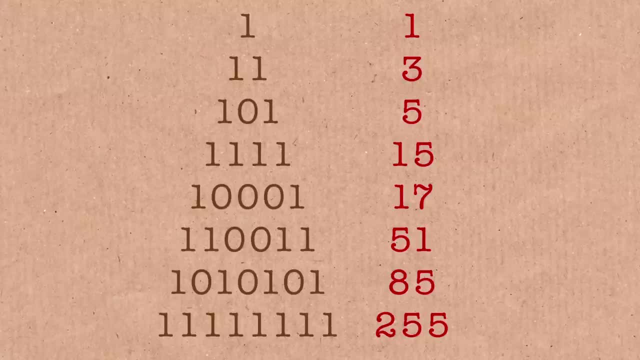 And here I'm going to stop and I'm going to look at what these numbers are. 3 is prime. 5 is prime. 15 is 5 times 3.. 17 is prime 51 is 17 times 3.. 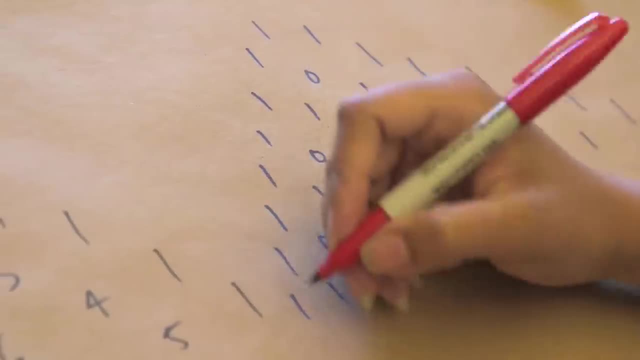 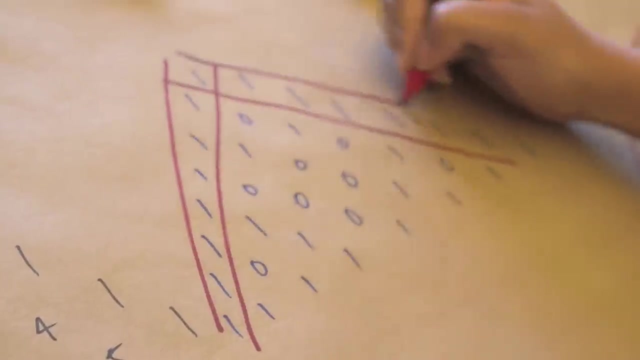 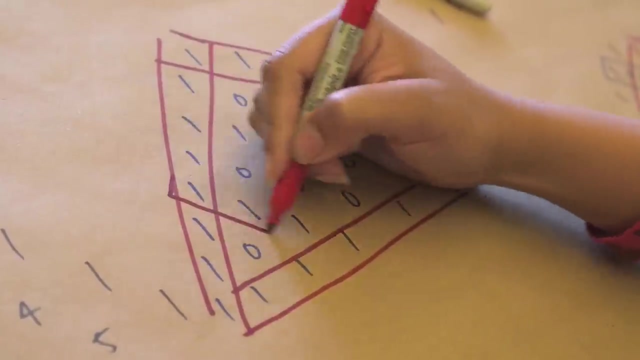 diagonals, that are all ones, and all of the rows, that are all ones. So I'm going to do this, which isn't the world's prettiest thing, but it's pretty nice, And this shape should maybe start to look a little familiar if you've played. 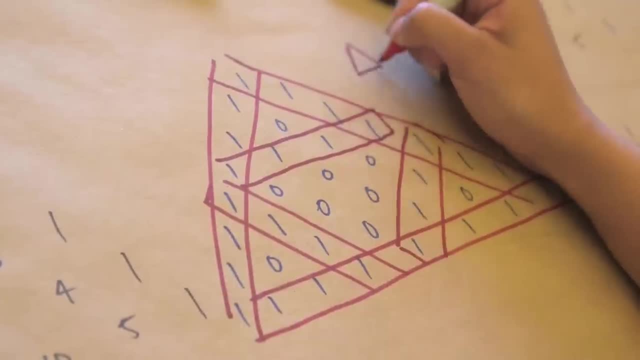 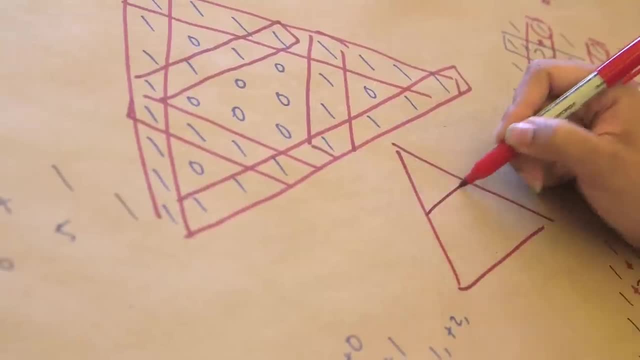 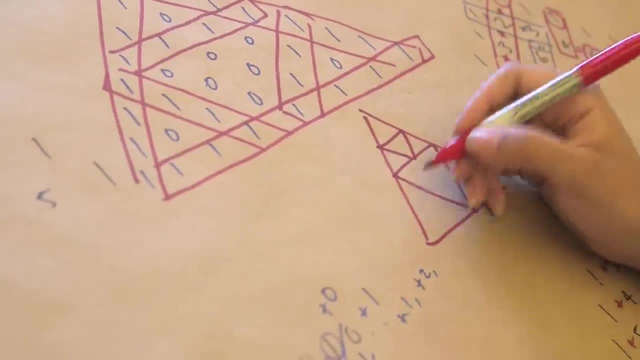 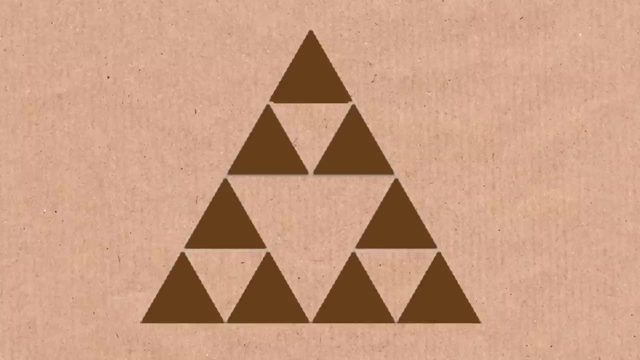 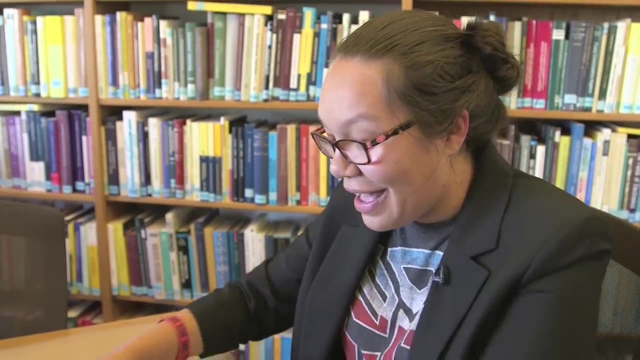 and then I can just keep doing this on all of the upward-facing triangles as many times as I want. So, yeah, this can just go on for a long time. And it turns out that the way that the evens and odds show up in Pascal's triangle, when I convert them to mod two, I can make Pascal's triangle. 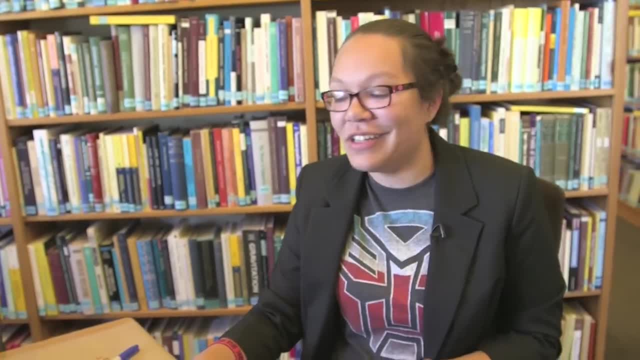 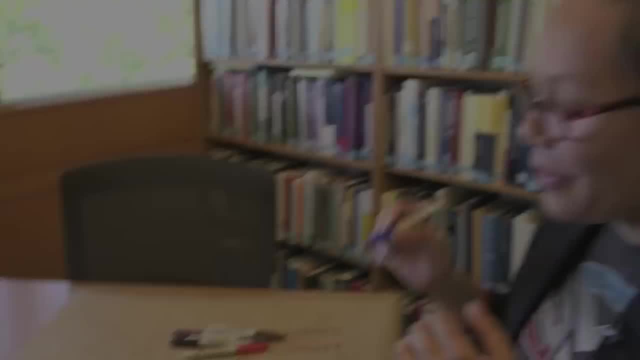 as big as I want, and I'm just going to keep getting iterations of Sierpinski's triangle. So that's really cool, That's awesome. That's really cool by itself, but it gets cooler using the mod two construction. There's something else we can do in mod two, though. In particular we can: 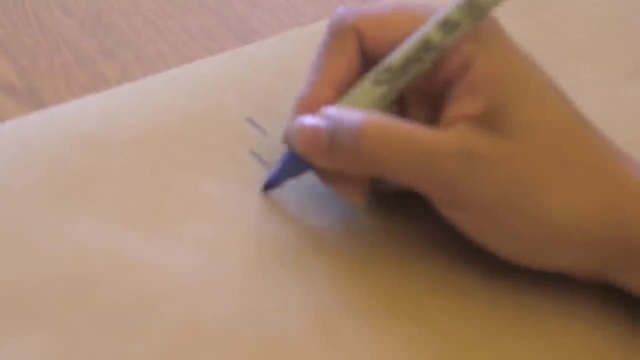 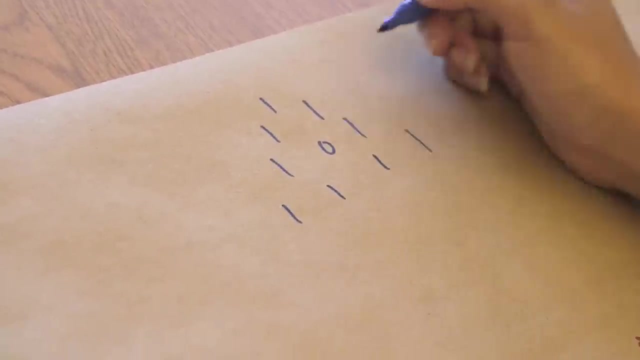 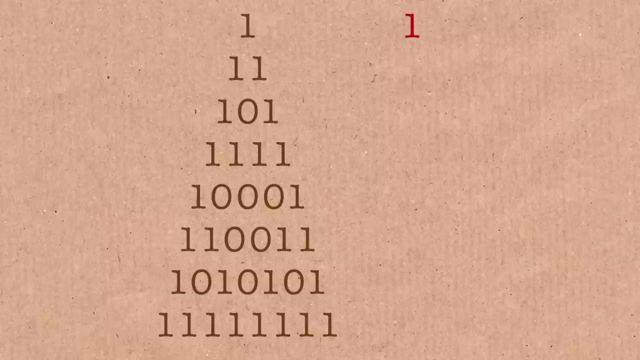 write down the same things, but let's write them now as we've got ones and zeros right And for most people, ones and zeros kind of remind them of binary. So let's just see what happens when we transcribe these from binary. You know, one in binary one And then one. one in binary is 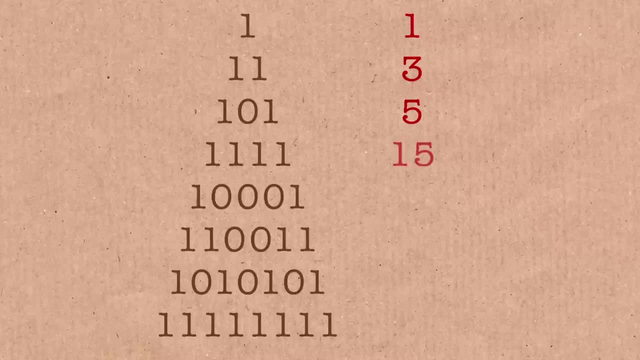 three: One zero one is five. One one one is 15.. And then the next one: one zero, zero, zero one is 17.. Now, these may not immediately appear pretty cool, But if I kept going, the next one. 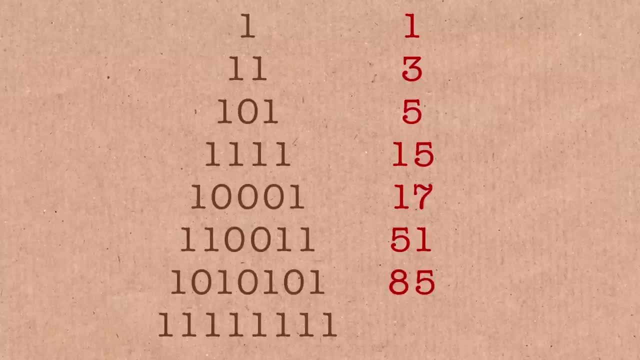 is 51.. The next one is 85.. After that is 255.. And here I'm going to stop and I'm going to look at what these numbers are. Three is prime. Five is prime. Fifteen is five times three. 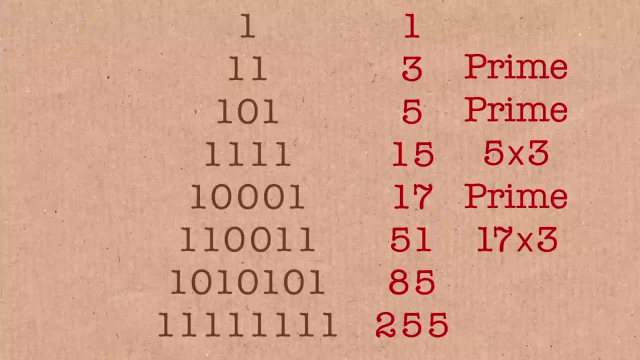 Seventeen is prime, Fifty-one is 17 times three, Eighty-five is 17 times five And 255 is 17 times 15.. So you'll notice that every time I get a prime, I go back and I just multiply by. 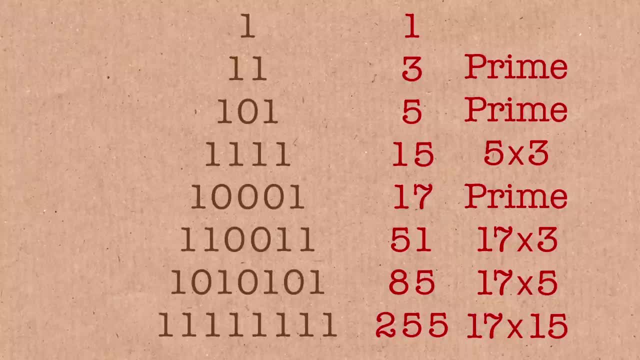 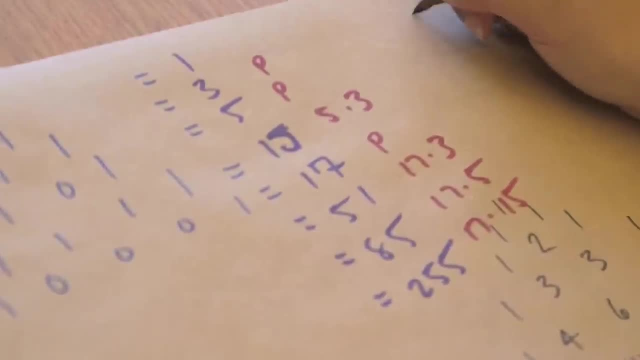 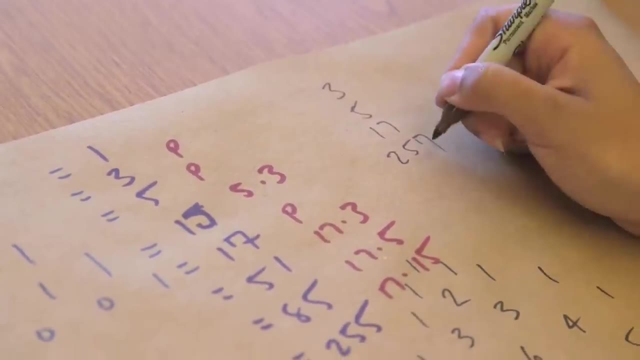 all the things that came before and I can generate the next, you know, n minus one entries. So the primes that we have here- actually at least the ones that I'm that we're certain of- are actually Fermat primes, Or Fermat primes rather, Which means that they can be written of the form two. 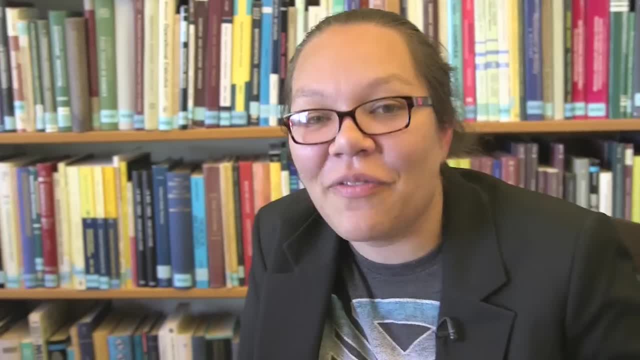 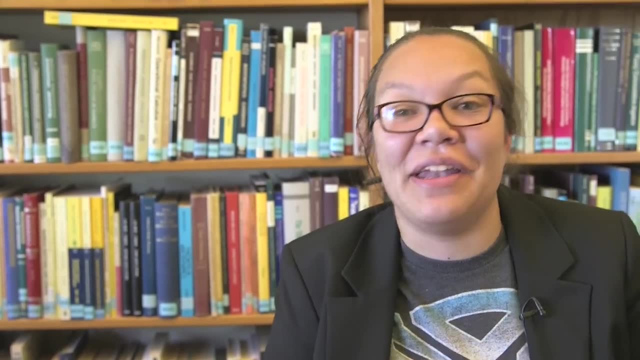 to the two, to the n plus one, Somehow, every time I talk to a mathematician. even ten minutes ago, when I asked a different mathematician for an idea, he told me something I'd never heard before. So, even if maybe somewhere out in the world, all of the things you couldn't do with this. 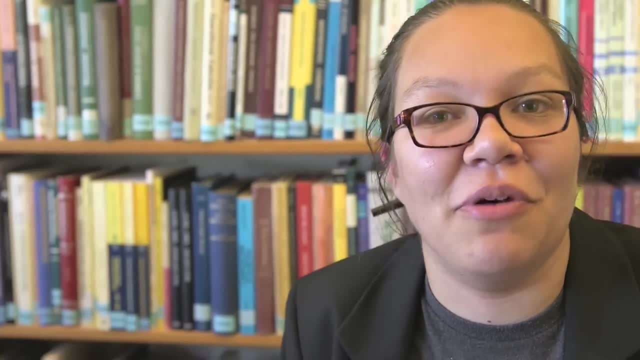 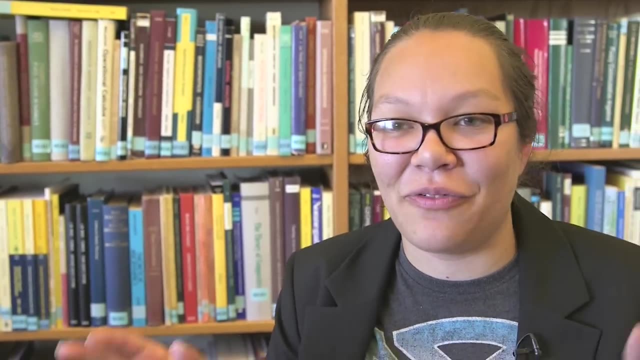 triangle are done. I don't know if there's any one person who knows them all, And maybe there's only one person who knows one of them, and we just have to keep exploring this triangle and seeing if we can collaboratively explain everything inside of it, But it's an infinite. 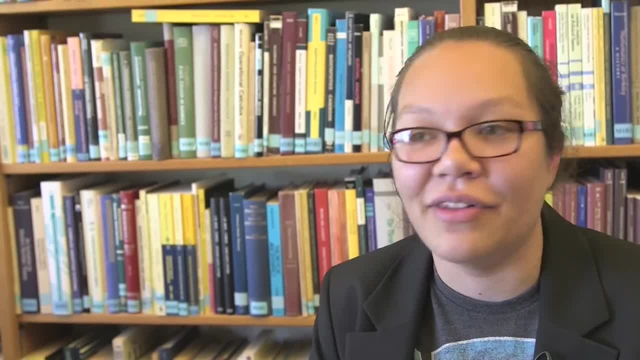 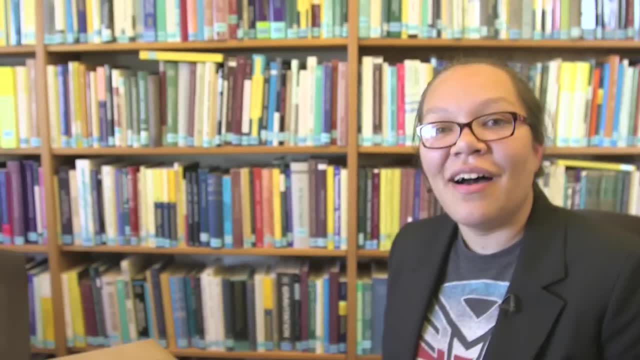 triangle, right, So maybe there are things on the hundredth line down that we haven't explored yet. I feel like it wouldn't be a Numberphile video if somehow the Fibonacci sequence didn't show up. So I'm going to show you where the Fibonacci sequence is in the past Scales triangle, because 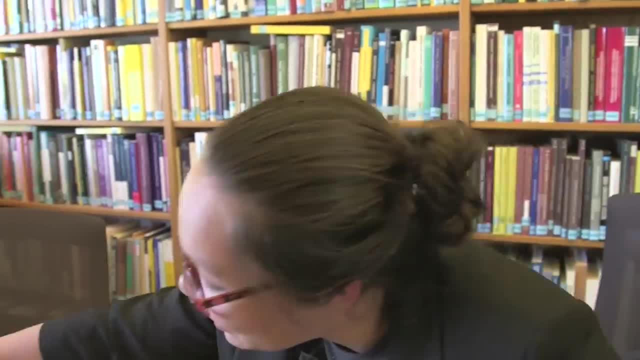 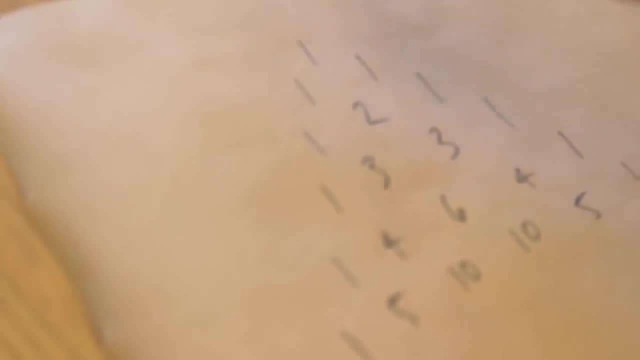 this is a Numberphile video. So what we're going to do is we're going to add up the shallow diagonals. So what that means here is the triangle kind of inscribes diagonals already right, Like I can look at this one and just kind of. 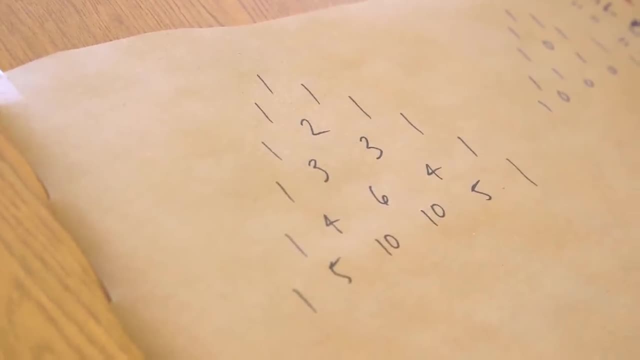 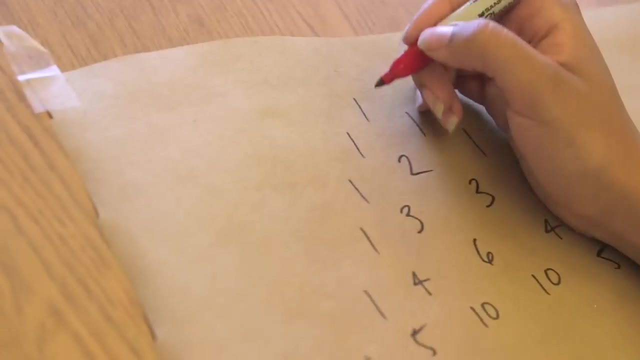 follow this. But a shallow diagonal means that I'm going to kind of go off at a slightly higher angle than I would have if I was just following the way I drew this triangle. So, for example, the first Fibonacci number is one, so that's my shallow diagonal. And then this one doesn't have 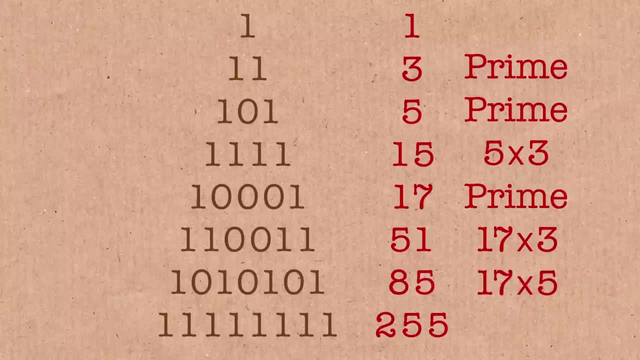 85 is 17 times 5. And 255 is 17 times 15.. So you'll notice that every time I get a prime, I go back and I just multiply by all the things that came before it and I can generate the next. you know, n minus 1 entries. 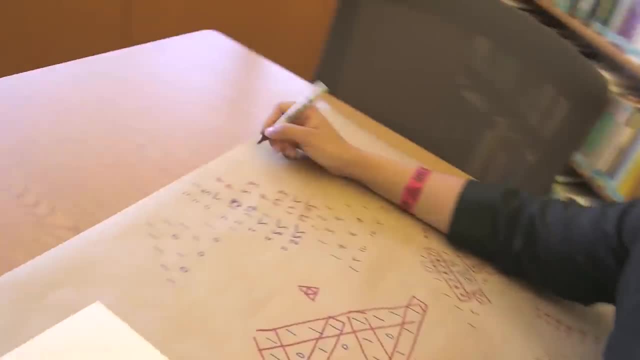 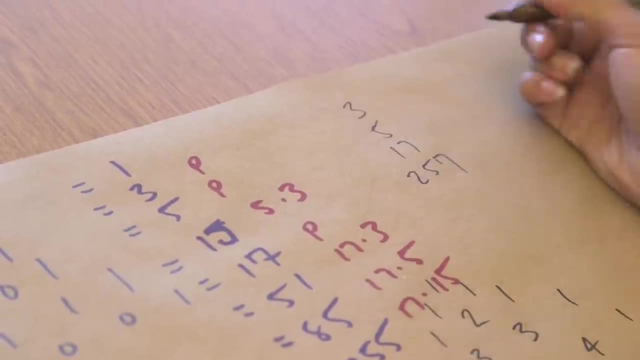 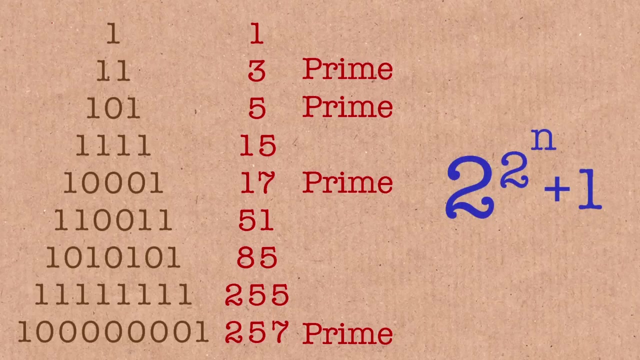 So the primes that we have here, actually at least the ones that we're certain of, are actually format primes, Right Or fermat primes rather, Which means that they can be written of the form 2 to the 2 to the n plus 1.. 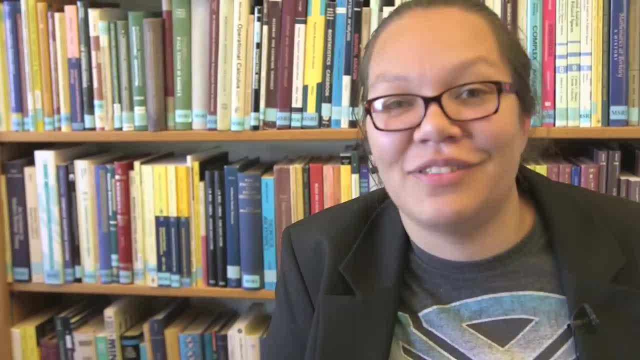 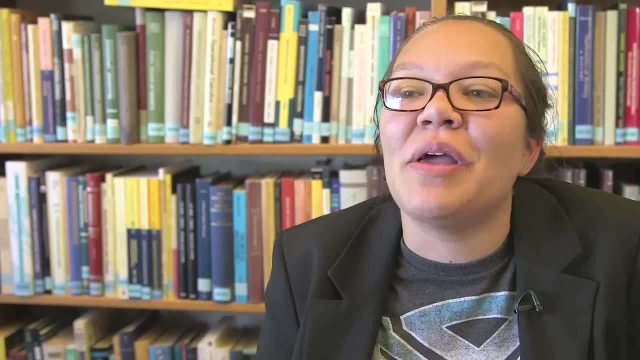 Somehow, every time I talk to a mathematician. even 10 minutes ago, when I asked a different mathematician for an idea, he told me something I'd never heard before. So even if maybe somewhere out in the world, all of the things you couldn't do with this. 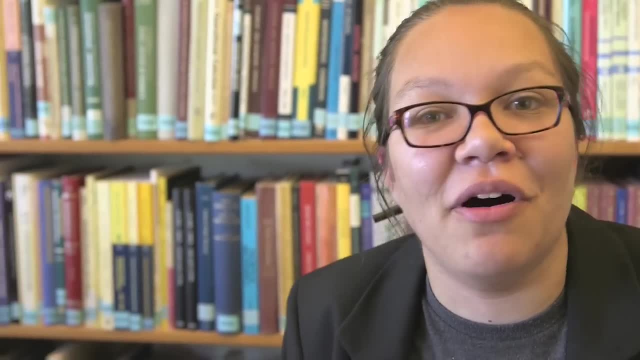 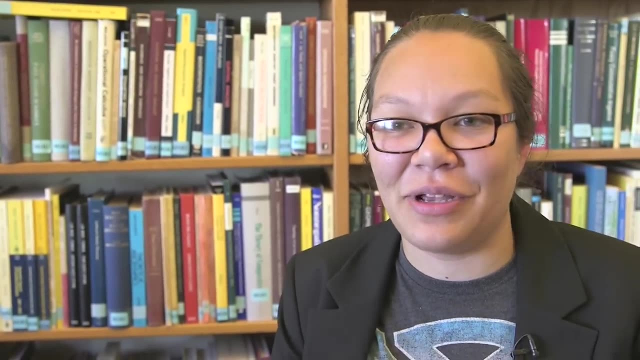 triangle are done. I don't know if there's any one person who knows them all, And maybe there's only one person who knows one of them, And we just have to keep exploring this triangle and seeing if we can collaboratively explain everything inside of it. 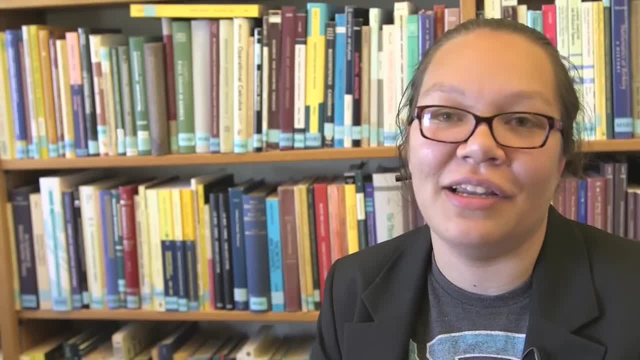 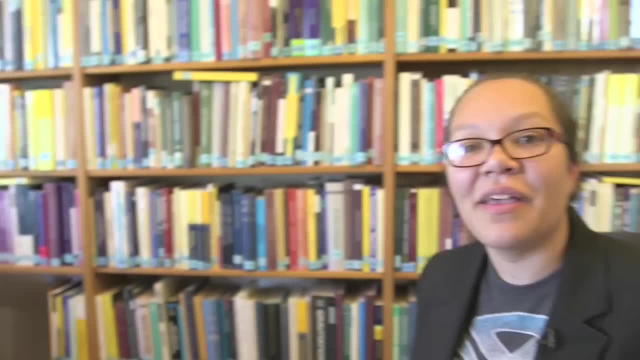 But it's an infinite triangle, right? So maybe there are things on the hundredth line down that we haven't explored yet. I feel like it wouldn't be a Numberphile video if somehow the Fibonacci sequence didn't show up. So I'm going to show you where the Fibonacci sequence is in the Pascal's Triangle, because 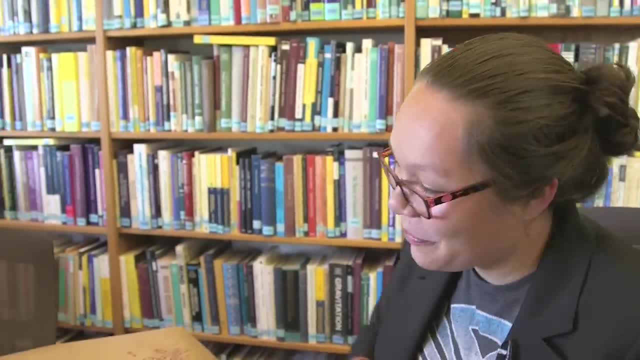 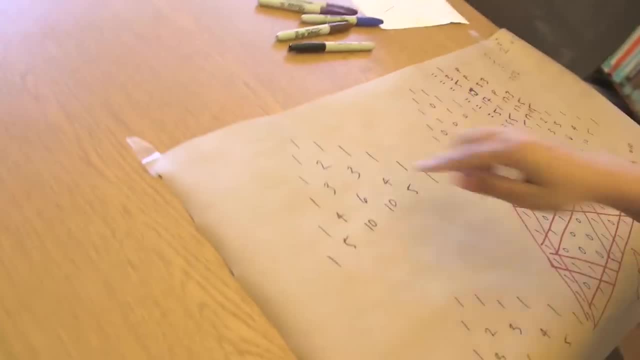 it's a Numberphile video. So what we're going to do is we're going to add up the shallow diagonals. So what that means here is the triangle kind of inscribes diagonals already right, Like I can look at this one and just kind of follow this. 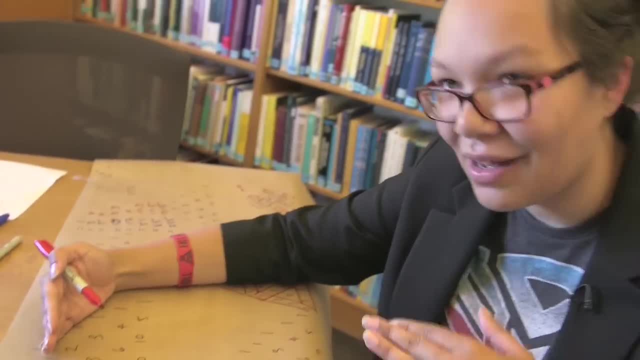 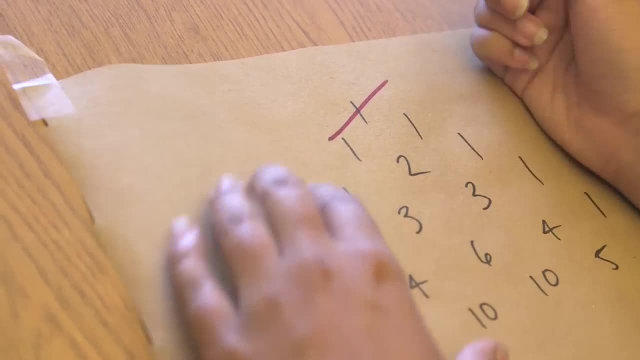 But a shallow diagonal means that I'm going to kind of go off at a slightly higher angle than I would have if I was just following the way I drew this triangle. So, for example, the first Fibonacci number is one. so that's my shallow diagonal. 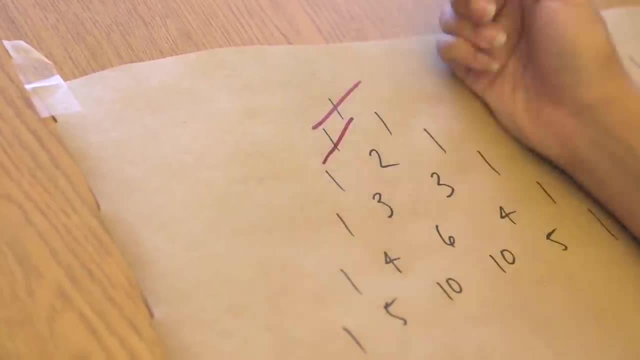 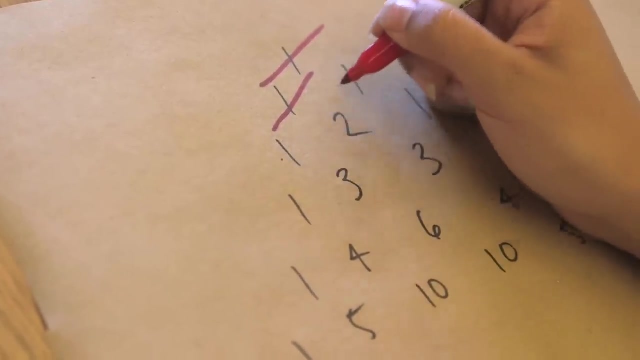 And then this one doesn't have any other shallow neighbors, so it's just by itself also. So now we have one one, Okay, So this shallow diagonal is a one and then this one. So we do this and we get two.